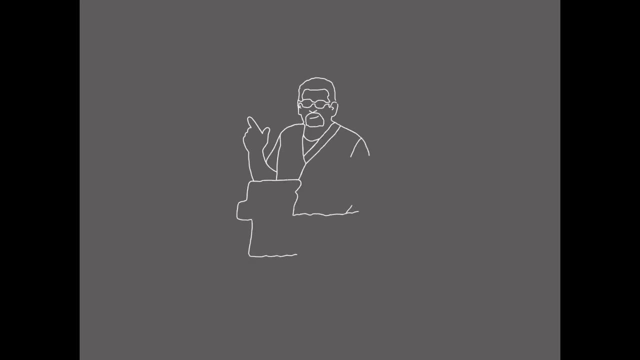 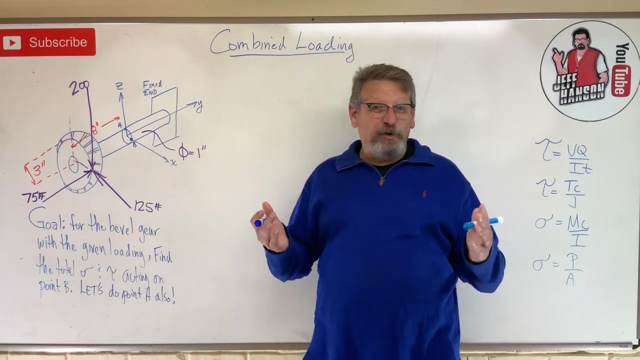 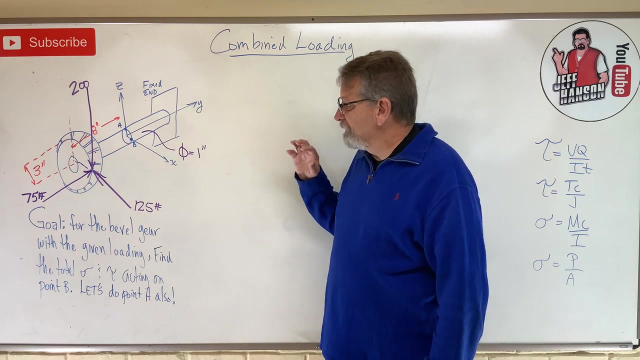 Hey gang, welcome back. We're talking about combined loads. I think it's one of the hardest things for my students to grasp is what's going on. There's so much going on on these combined load problems. okay, Like this problem here. I've got a shaft coming out from a wall with a gear on. 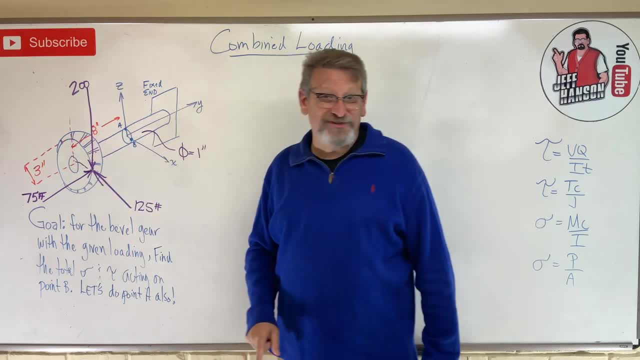 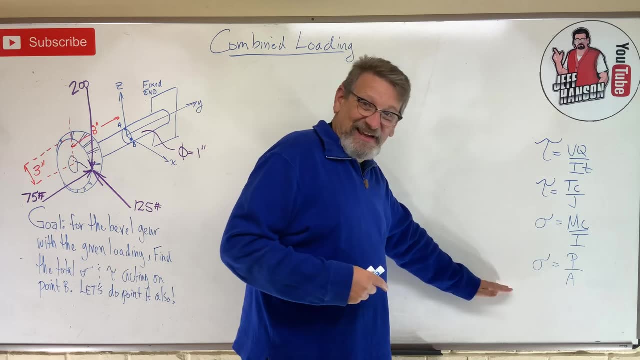 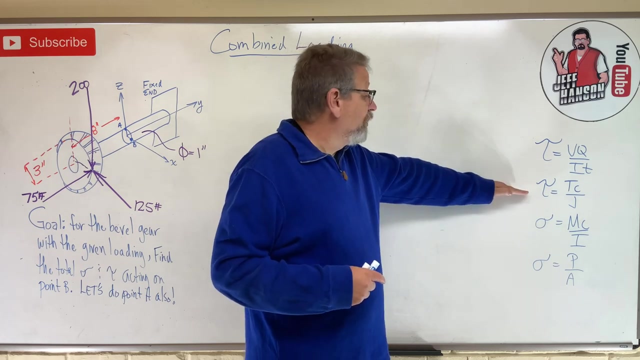 the end of it and it's got one, two, three different forces on it. The thing about combined load problems is that one force can cause all of these things right. One force can cause shear stress- vicot right Shear stress. It can cause torsion, twisting TC over J stress. 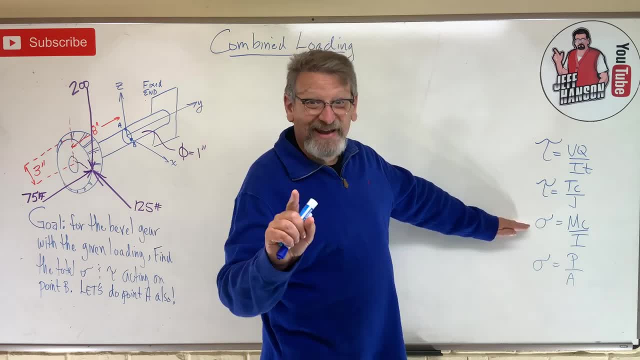 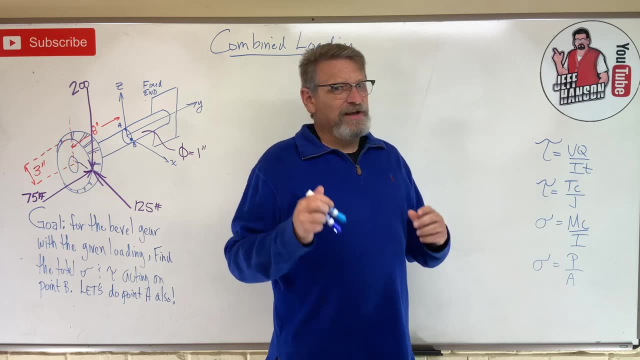 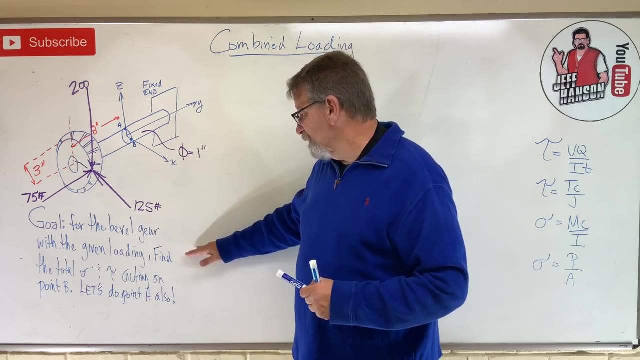 In the normal stress department. it can cause MC over I bending stress, And then also it can cause P over A, just compression or tension stress. And so for everything we're going to do, like for this problem, find for the bevel gear with the given loading, find the total sigma and tau. acting on point B. 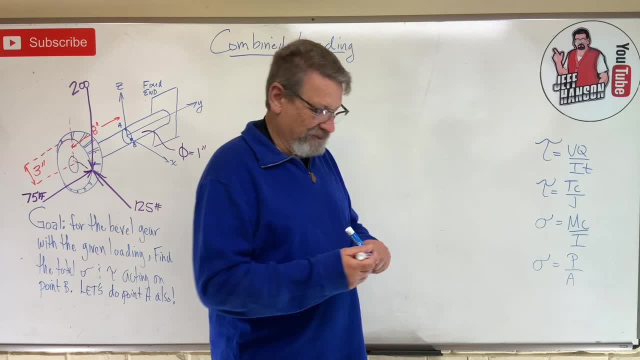 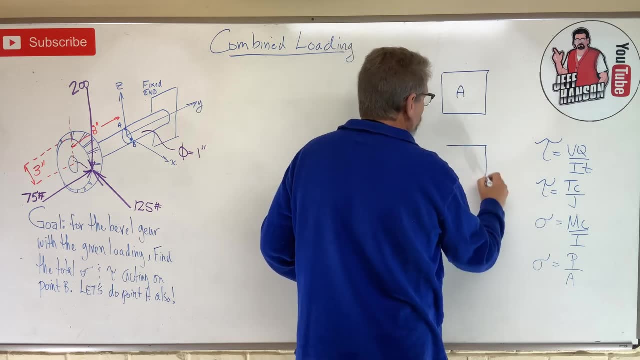 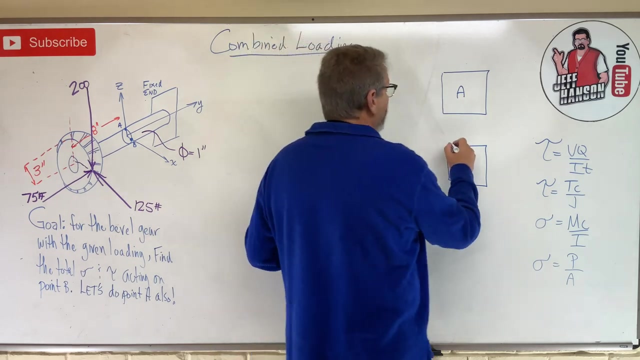 And it says, hey, while we're there, let's do point A too, okay, So what we're going to do is this: okay, These are my stress elements. Remember stress elements? Okay, We got to find the stress element for A and the stress element for B. What's that going to look like? It's going to look like: 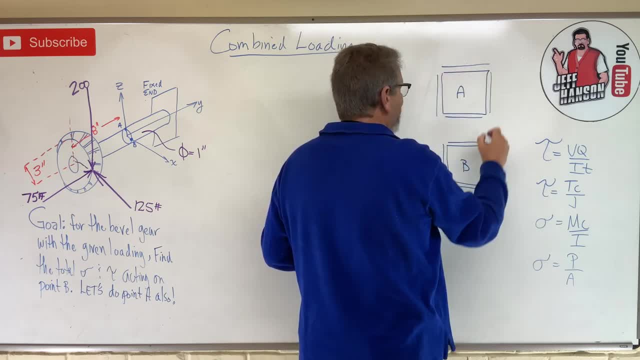 this: okay, There's going to be shear stress and then there's going to be normal stress. Uh-oh, I'm overlapping here. No, Okay, there you go. right, We got to find out which way the arrows go on these stress. 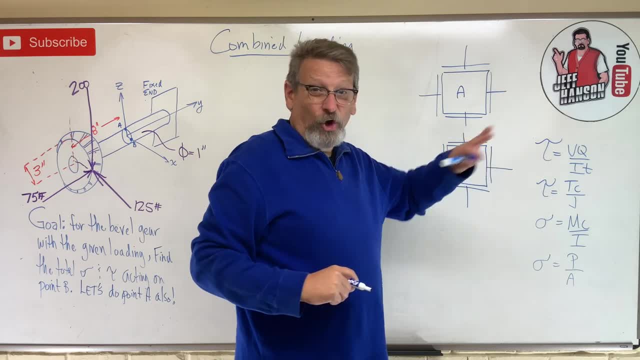 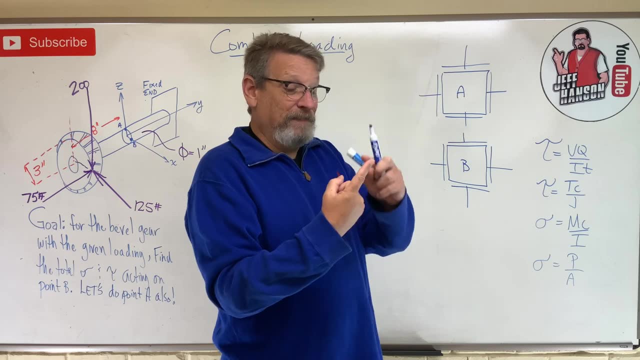 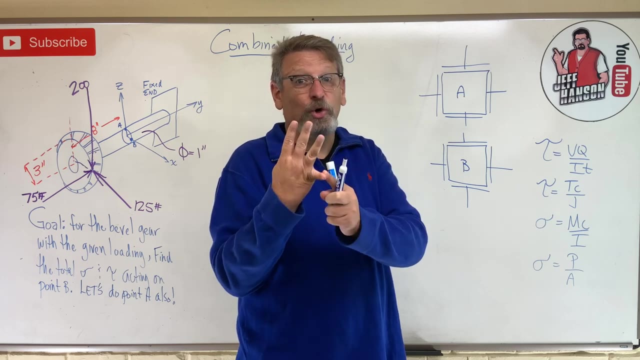 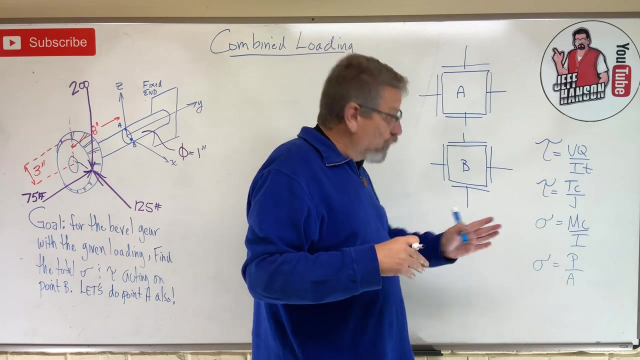 elements and how big the components are. okay. So for any one force, right, Every single force- can cause bending, compression or tension, shear or tension, And then there's going to be shear stress. So we have to evaluate each force for all four of those things. There's one more thing that could. 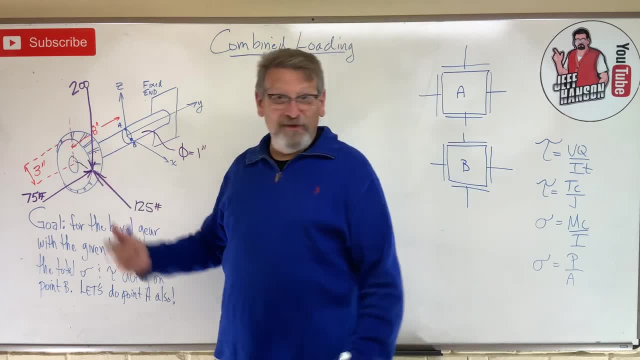 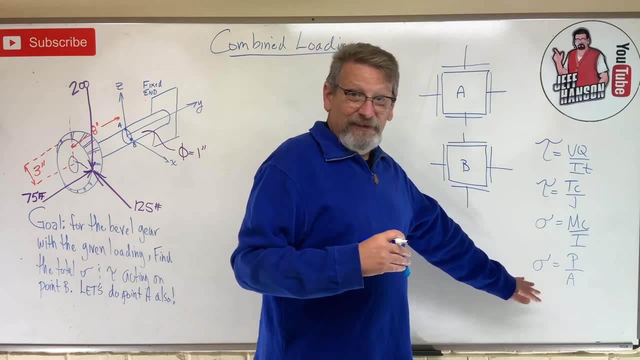 be over there and this could be a hollow pipe that we pressurize with pressure. Then we'd have PR over T and PR over 2T also. But luckily this isn't one of those problems, okay, So let's see. 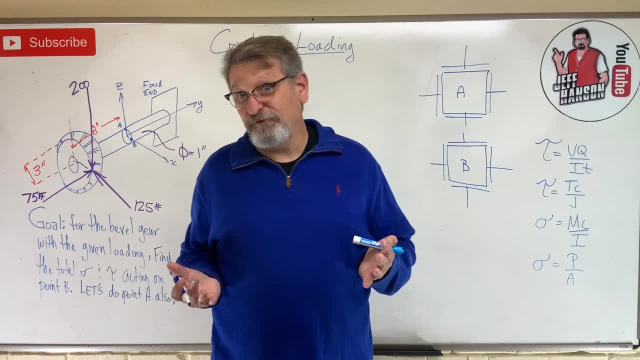 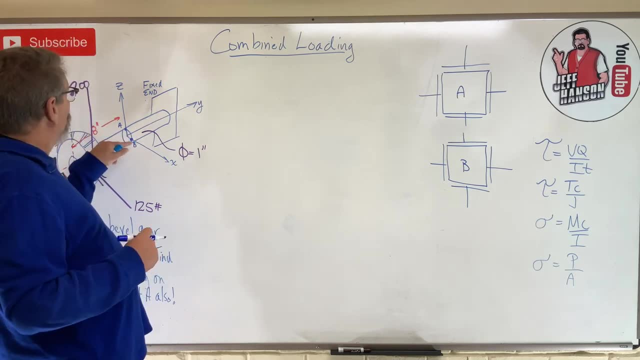 if we can do this. I'm going to show you how I think about it and see if that helps us solve this. okay, So the first thing I like to do is draw the cross-section of the force. So I'm going to draw a cross-section that I'm interested in. So I'm interested in this cross-section. 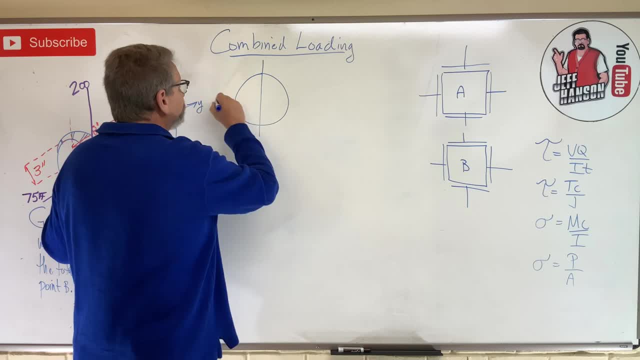 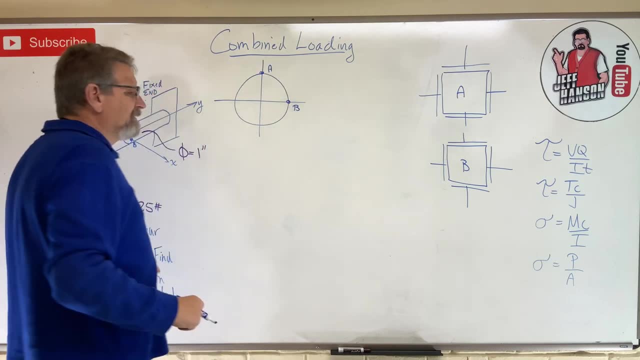 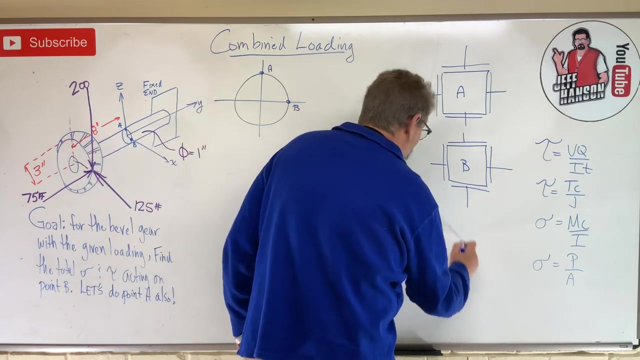 right here and I've got this, And I've got here's point B and here's point A. okay, And what I'm going to do is this: This gets a little bit confusing because there's a lot going on here, but what I'm going to do is this: I always want to draw these cross-sections. 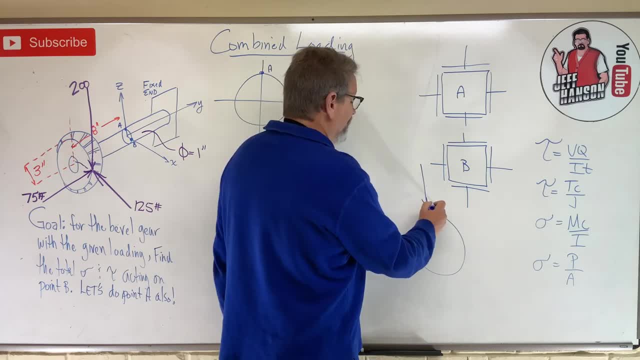 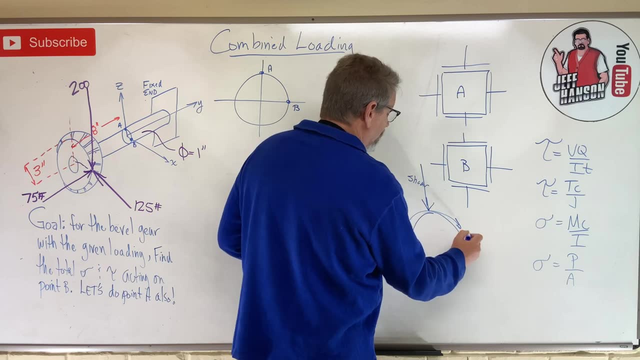 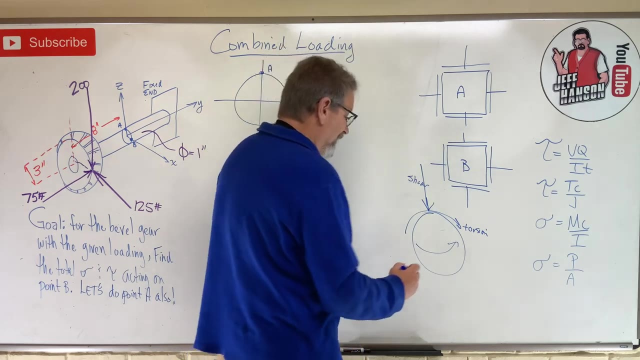 I'll draw this: okay, That just an arrow down means shear. okay, That means shear here. If I draw this, okay, that means torsion. If I draw this across the middle, that means that's a bending moment, okay. And then, right in the center of the circle, I'll either draw a plus: 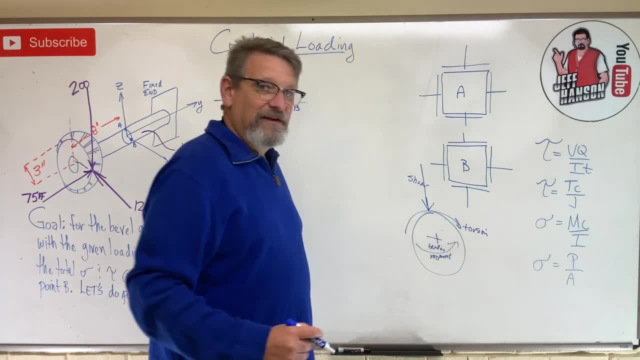 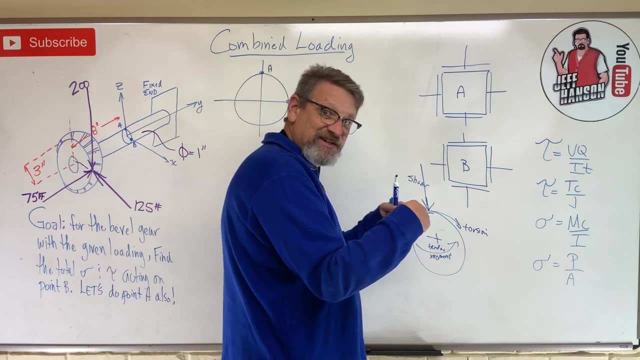 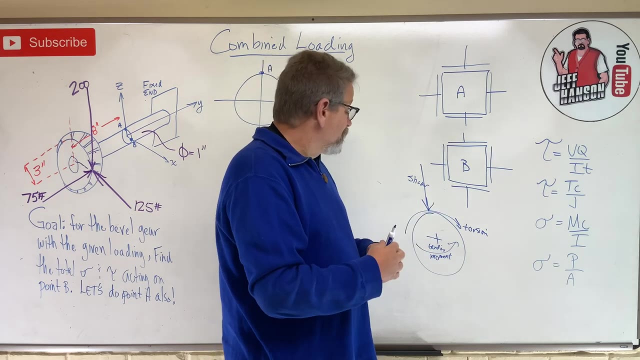 or I'll draw a minus, okay, And that to me indicates that there's either a force pushing, which would be a minus, right, Because compression is negative, or a plus, which means that there's just a P over A. that's making the shaft longer, right? So this is my P over A stress. this is my. 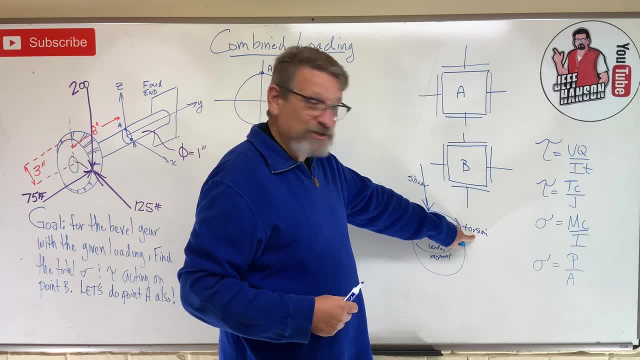 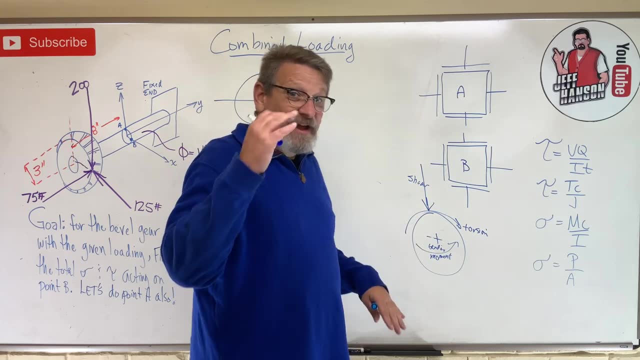 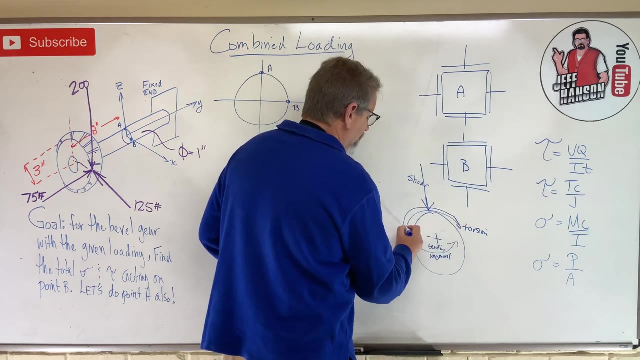 MC over I stress, that's my TC over J stress and that's my VQ over IT stress. Now, I'm going to do these things For every single one of the forces acting on this, because what happens if I have this right? 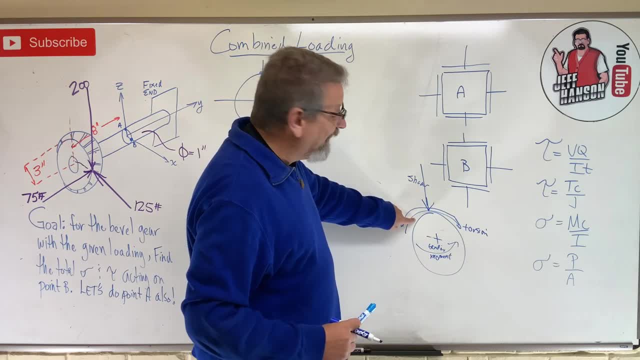 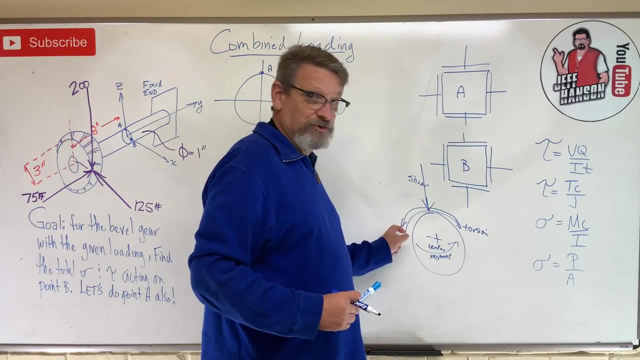 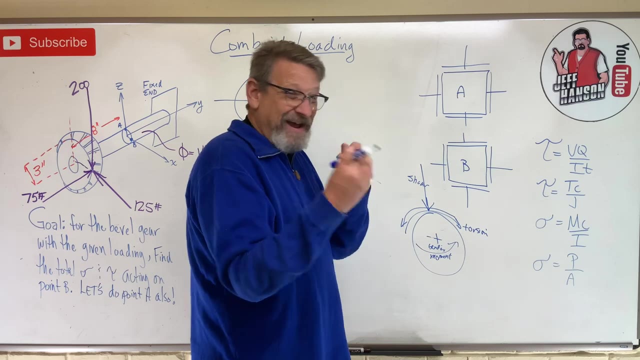 What happens if I have that? Well then I can take this one and that one and add them together and find out what is the resultant of those two torsions. right, Because I might have one that makes me spin clockwise and one that makes me spin counterclockwise. but when I add them together, 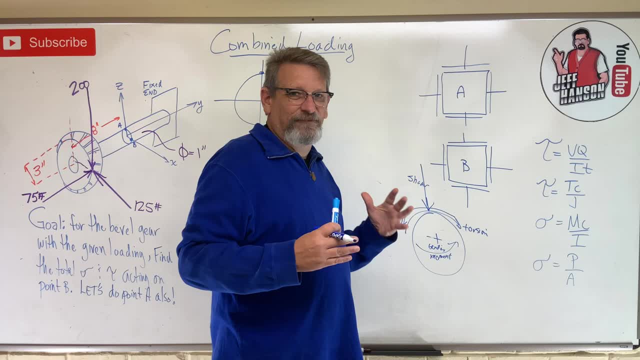 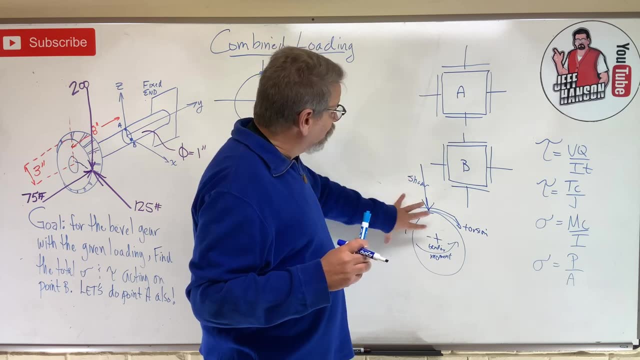 my net is still a counterclockwise right, So I just need to find out what that net is. So there's going to be a lot of arrows going on, especially with three forces, and I'm going to draw kind of this diagram that has shear on it. 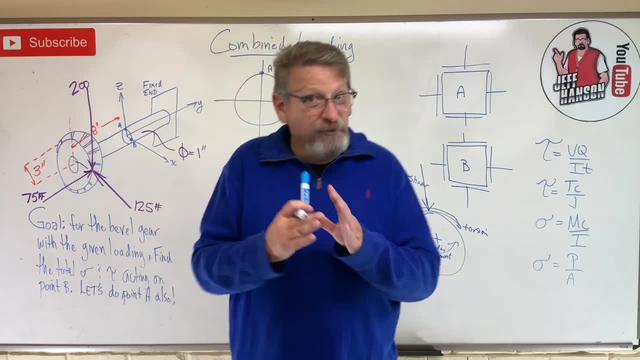 that has torsion, bending and compression. okay, So that's what I'm doing. So I'm going to go one force at a time and let's see if we can do this. okay, So there's our cross section. 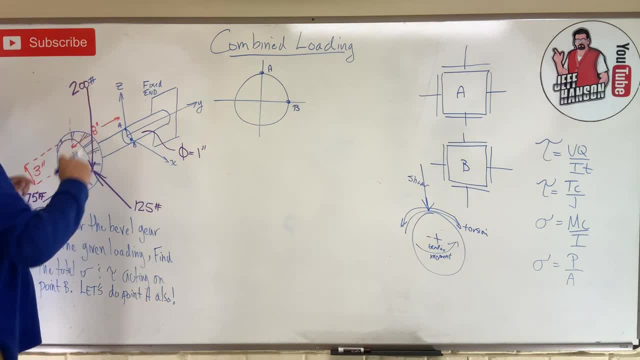 Let's start off with this guy right here. 200 pounds, okay, 200 pounds. what's he doing? Well, okay, number one, he's going to be doing a cross section. Number one: on that cross section does he cause shear, which is just a downward force. 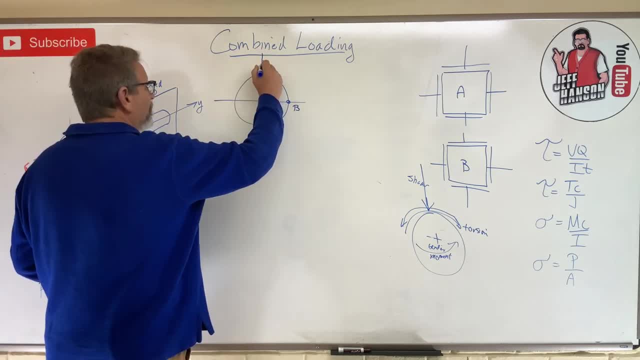 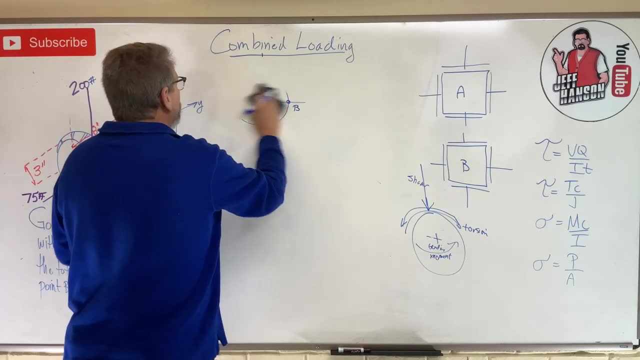 Yes, So up here, I'm going to do this. I'm going to redraw this higher up or be lower down. Let me give myself a little bit more room here. I'm sorry, I apologize. Okay, here we go. Okay, so here's the first one. is this guy right here 200 pounds? okay, He definitely causes that. 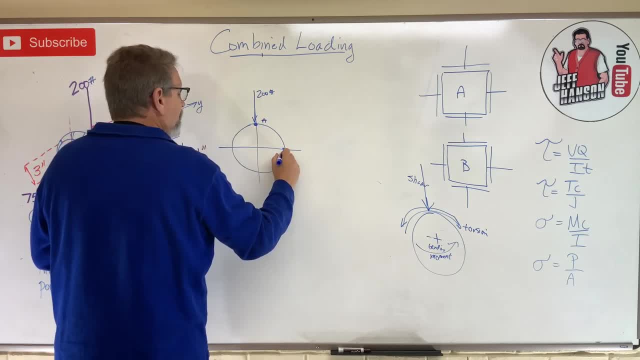 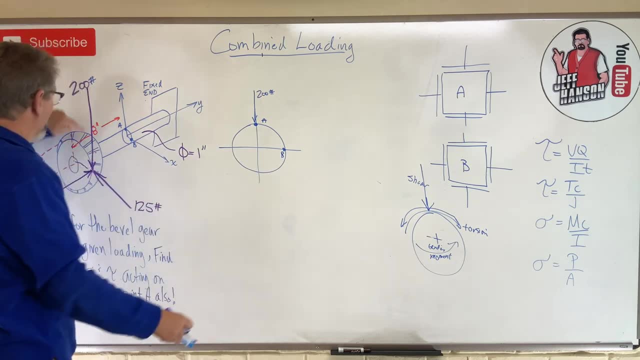 Here's point A. here's point B. okay, What else? What else does the 200 do? okay, Does the 200 cause torsion? Well, he's out here on the perimeter, so, yeah, he's going to make me spin this direction. 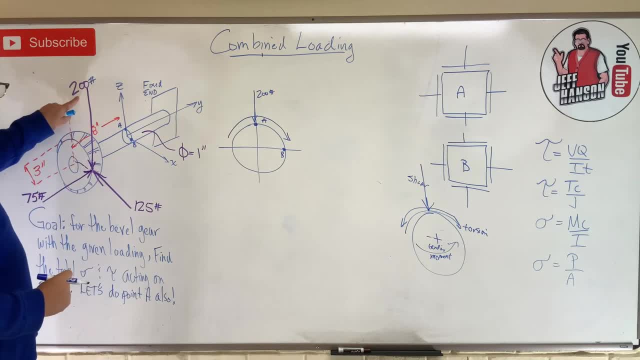 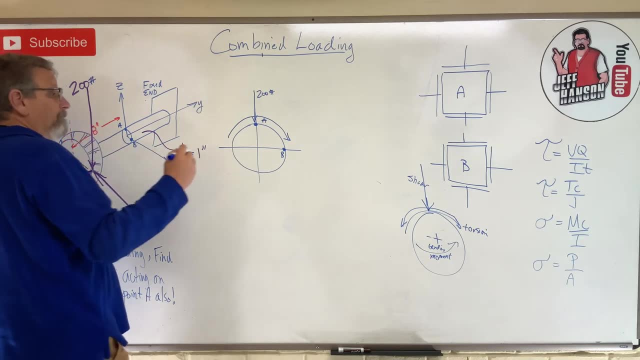 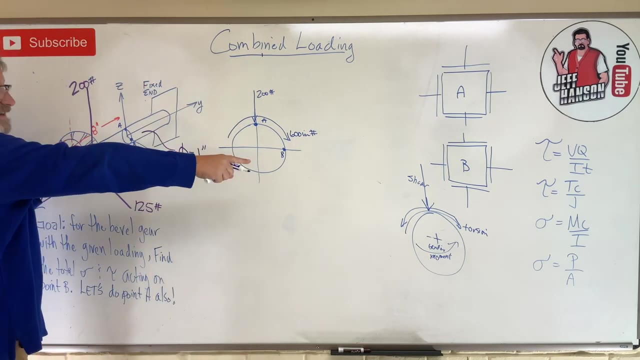 here, isn't he? And how much torsion is that? Well, it's force, times, distance, and the distance is this: radius, three inches. So 200 times three is 600, inch pounds. okay, Let's go to the next thing down there. Does he cause bending? Does the 200? 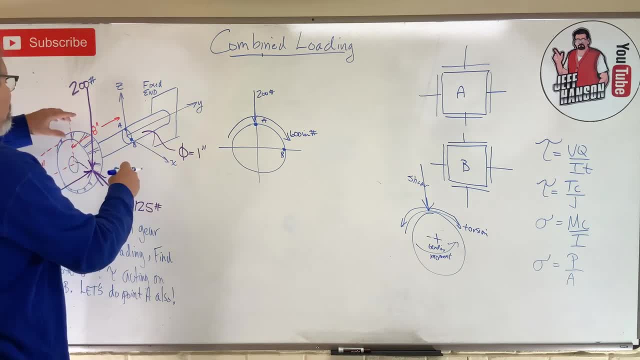 cause bending. Yes, right, It's the force that's making this thing. the 200 is making the whole thing bend downwards. right, Point A being on the top. he's going to be in tension, isn't he? So I'm going to say that this is 200 times eight inches right, Which is 1600.. I'm going to do this. 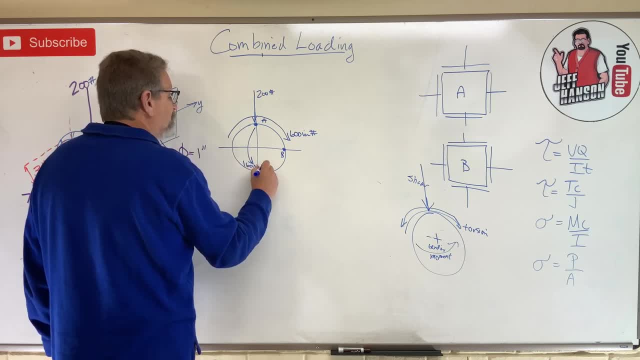 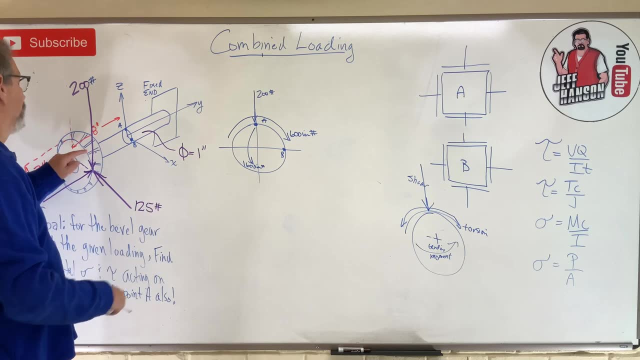 Okay, 1500 inch pounds. There he is, okay. What else is he? Is he causing compression? P over A stress? No, he is not causing any compression. okay, All right, so that's got him. Let's go to the next. 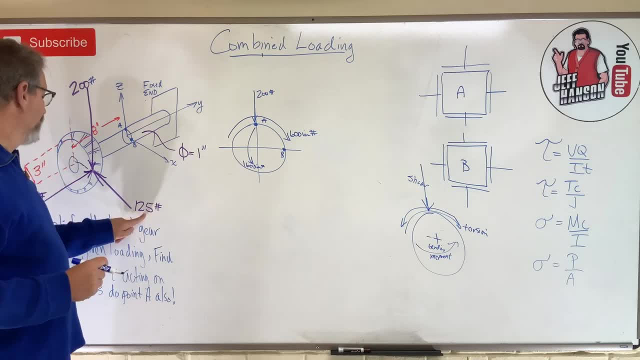 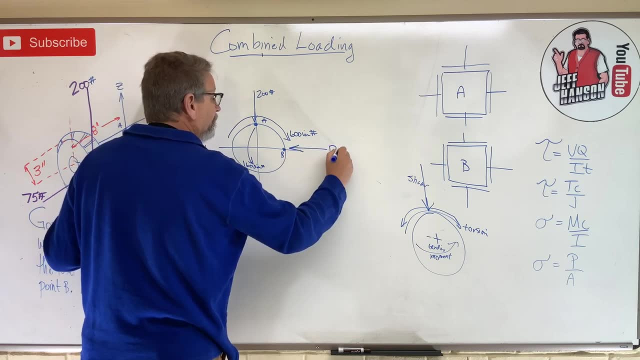 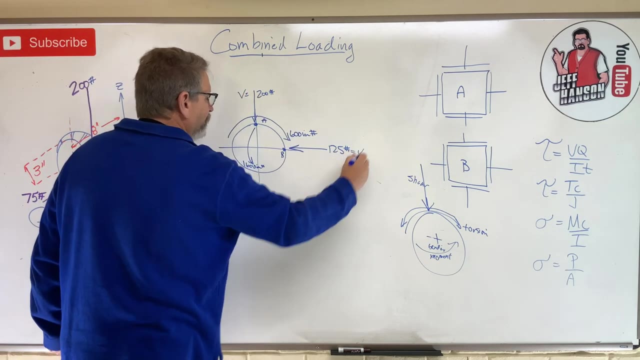 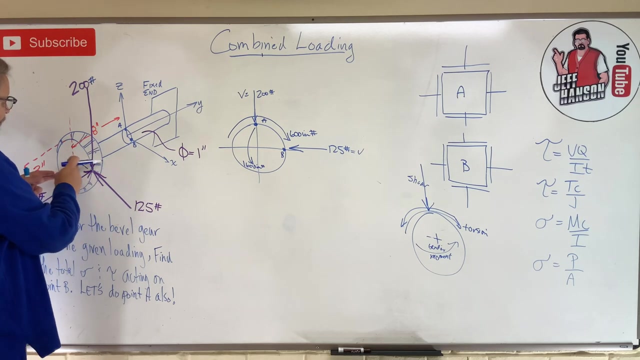 guy the 125.. Does he cause shear? Yes, and it is 125 like this. okay, And that shear is V, right, This is like V equals, V equals the shear force, right? Next one: does he cause torsion? Well, since he's pushing right on the center. 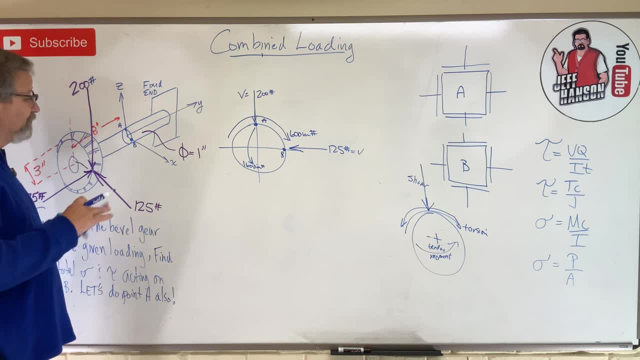 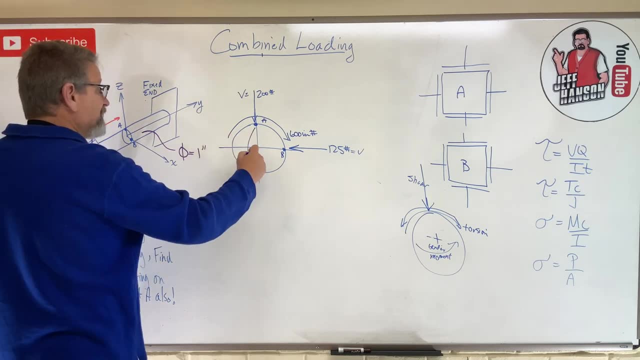 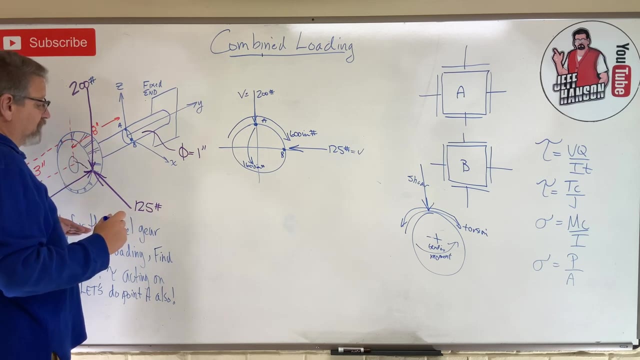 of the shaft? the answer is no. no torsion, okay. Does he cause bending? Yes, but not in the this direction here, but in this direction here, right. So he causes bending 125 times eight. What's 125 times eight? 800 plus 200 more, it's a thousand, isn't it? Okay? So it's going to cause. 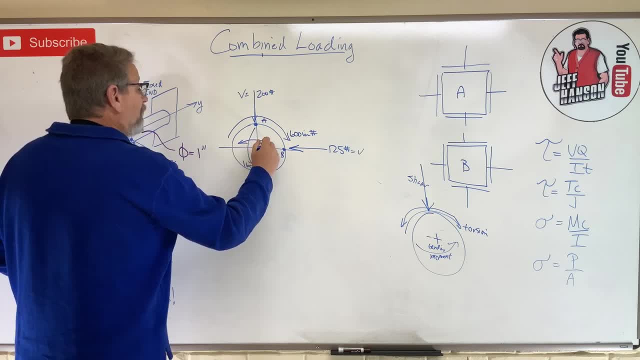 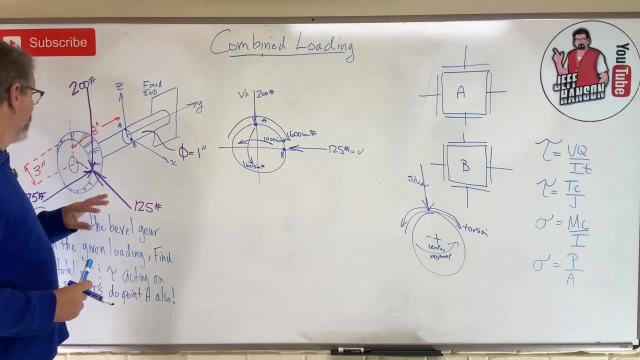 like this: 1000 inch pounds. okay, There's a lot of stuff going to be going on in my little diagram here, but we're going to figure it out okay. So a thousand. Does he cause any P over A stress? 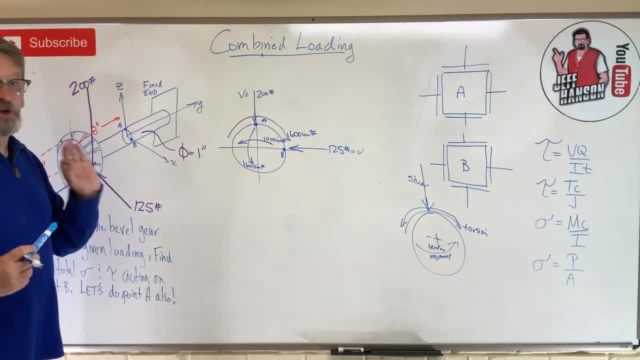 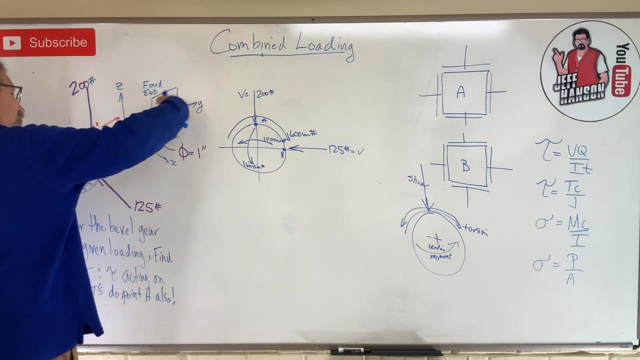 Does he cause any compression? No, it does not, okay. Okay, so that's got the 125, one more to go, the 75.. Does the 75 cause any shear? No, because he's just doing a compressing act there, isn't he Right? He's just causing that. 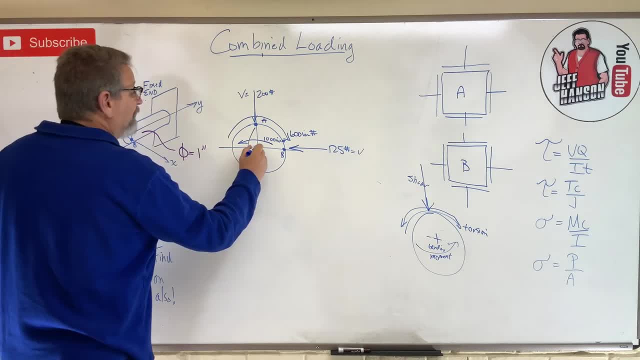 bottom guy, another P over A and it's compression. So right here in the middle I'm going to put a big minus right there in the middle, right From the 75,, 75,. okay, Does he cause any torsion? 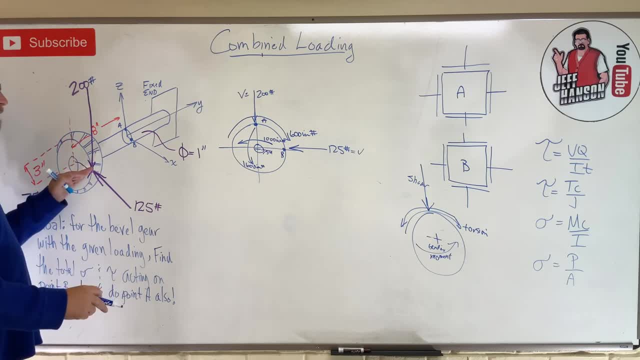 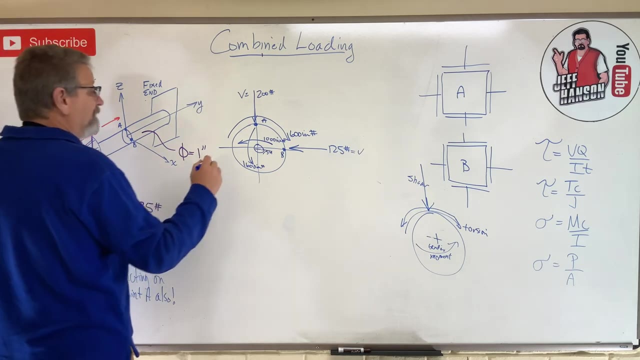 Well, no, he doesn't cause it to twist at all. Does he cause any bending? Yes, If it was pushing right in the middle, the answer would have been no, but since it's pushing off on the perimeter, there's a little bit of a moment right, And that little bit of a moment is actually going. 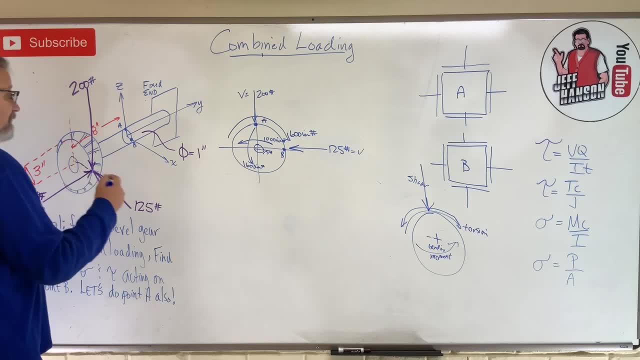 let's see. let's see. that moment is going to be going this way, isn't it? Zoop, Okay, Where this one caused that that shaft to bend into the board, the 75 causes it to bend out of the board, okay. 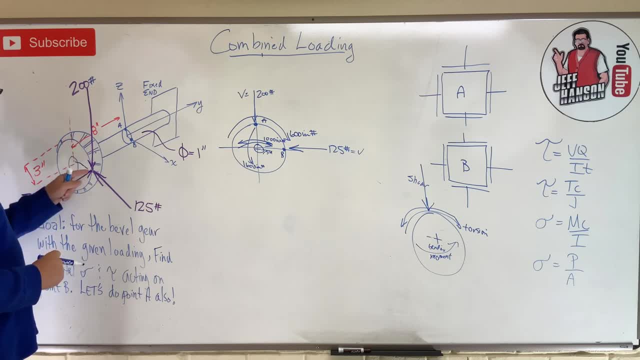 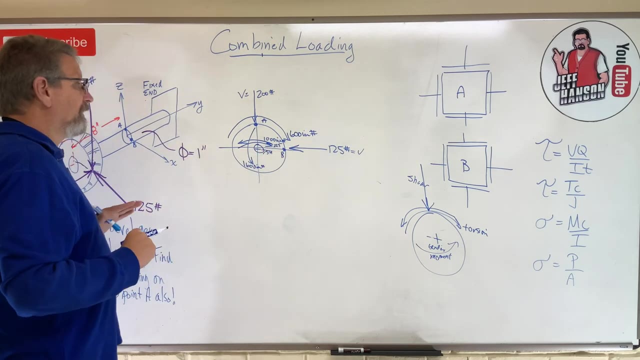 Now, what's the force? The force is 75, and what's the distance? The perpendicular distance is only three. okay, So 75 times two is 150, plus another 75 is 225,, 225,. okay, Are you with me on this? 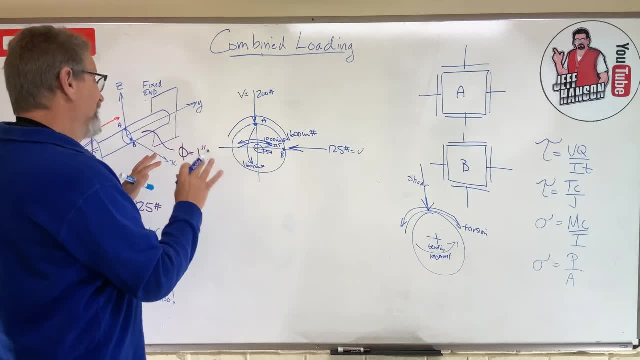 There's a lot going on here, right? I'm going to leave everything the way it is, except for one thing, and that is I have these two bending moments. I have one going this way and one going that way, right. 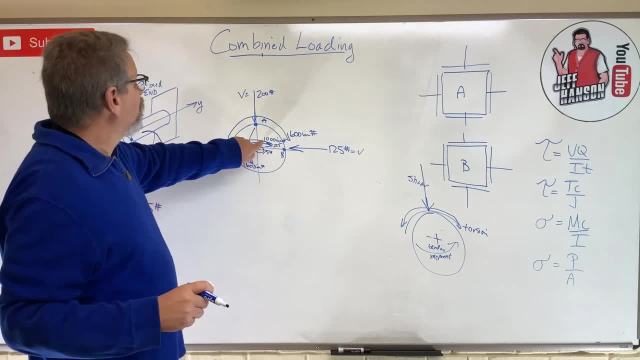 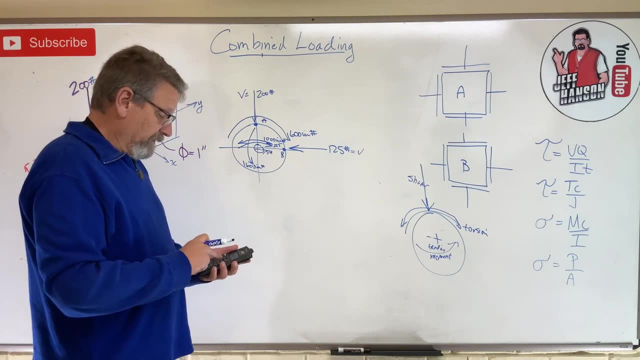 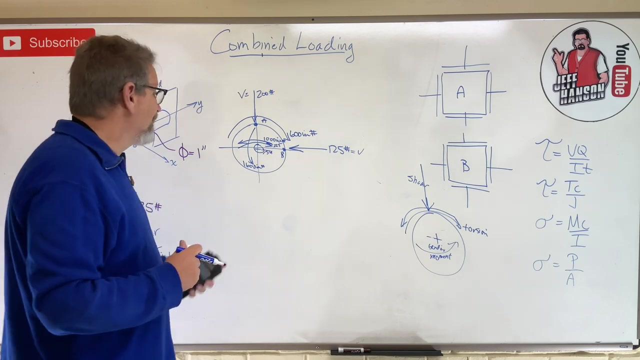 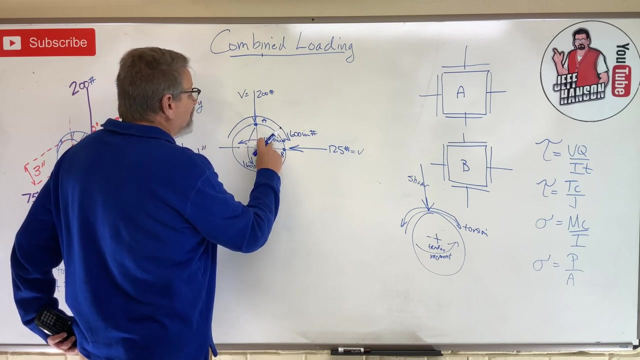 And so what happens is is this bottom one here just winds up taking off of that top one right. So if we take, if we take on clear, if we take a thousand right and we subtract from that 225, we get 775.. So let's just erase this bottom guy down here, okay, And let's turn this top guy. 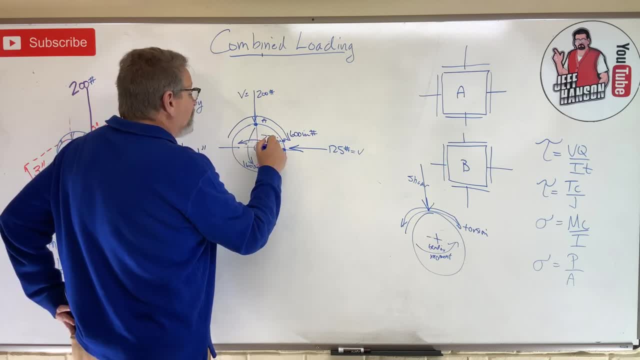 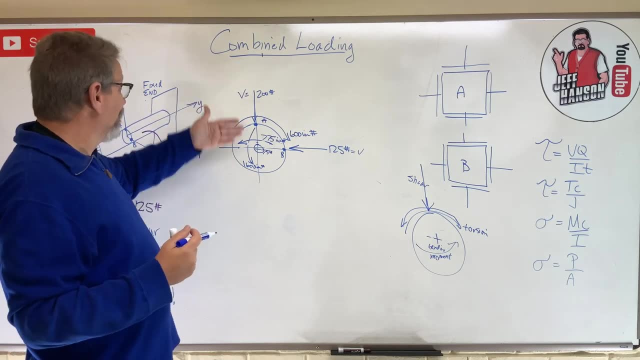 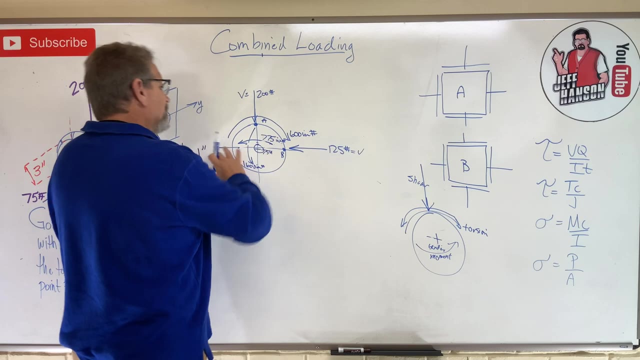 into 775, okay, You understand what I, what I did there. I just combined them. It's combined load and we just combined the load. Hey, hey, hey, Okay. so there's a lot going on this graph. I got shear force, I've got torsion, I've got bending this way and that way, and then 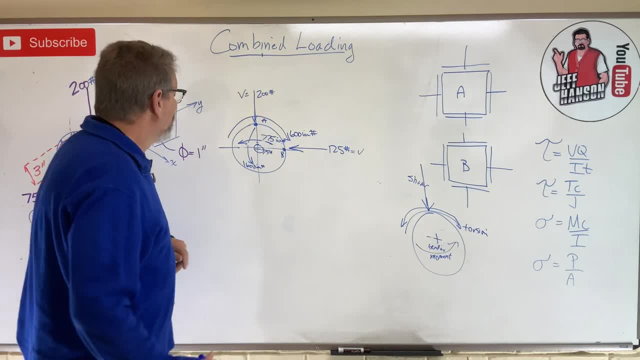 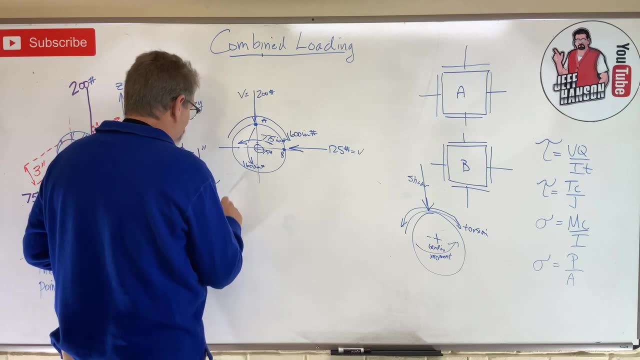 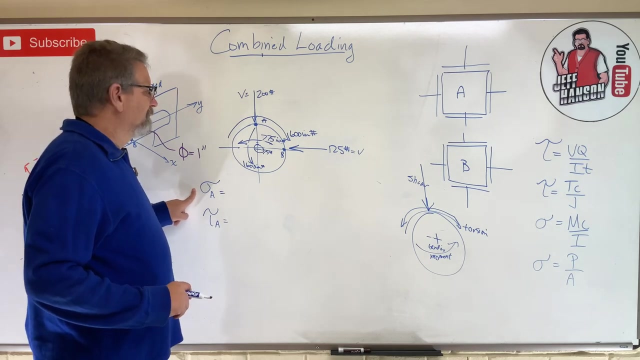 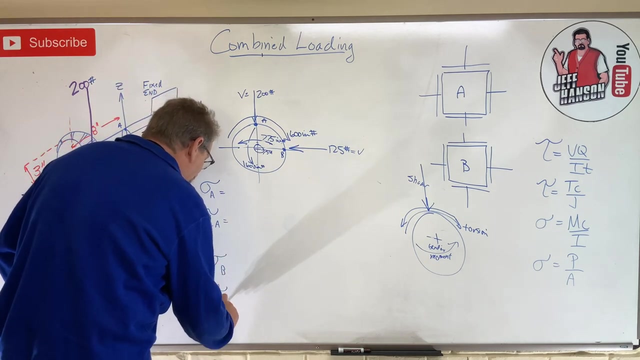 I've got compression, So let's go. okay. Let's talk about point A. okay, We got two things to do. We got sigma A and we got tau A. okay, So sigma A is point A being compressed. Yes, everything is being compressed, right, We got sigma A. here's sigma B: tau B. 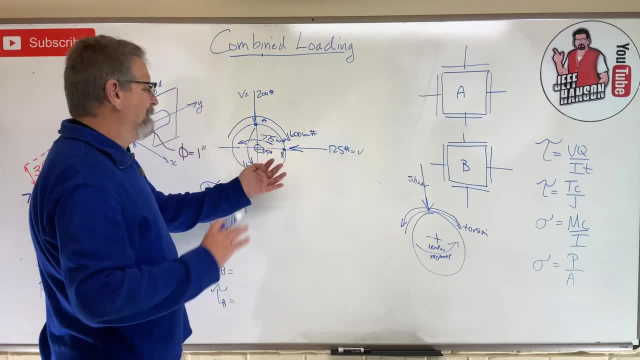 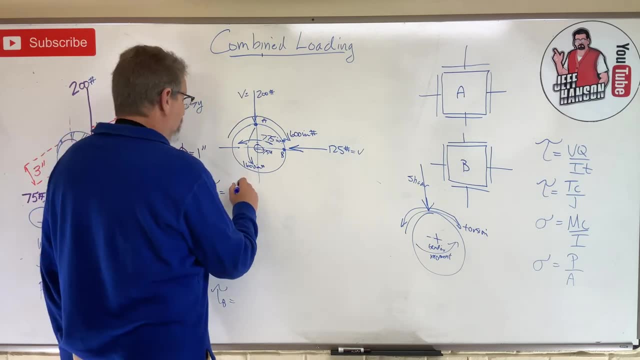 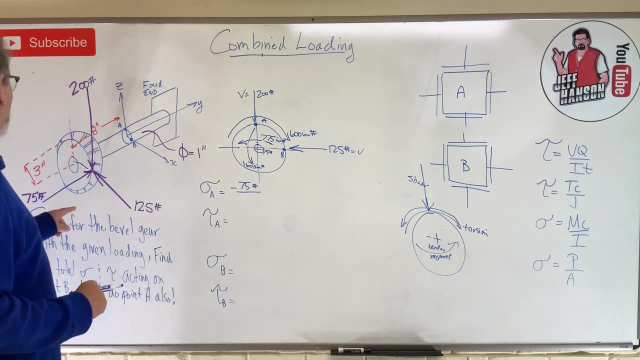 okay, So A and B, both are being compressed from the 75, right? So that's going to be negative P over A 75.. 75 pounds divided by oh, what's the area? What's the area? How big is that? Where is it? 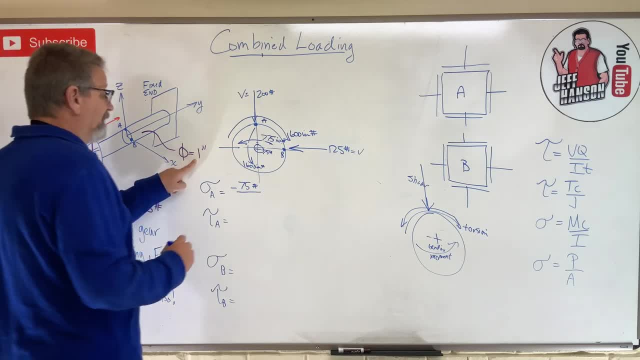 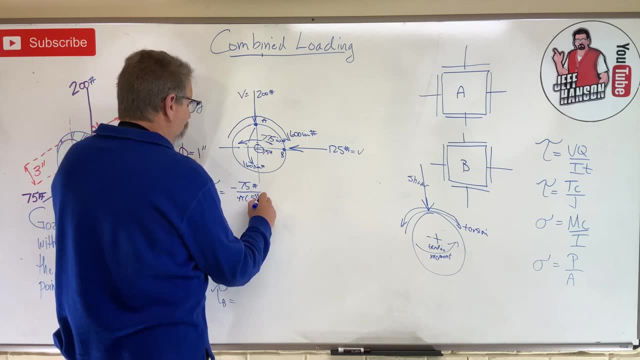 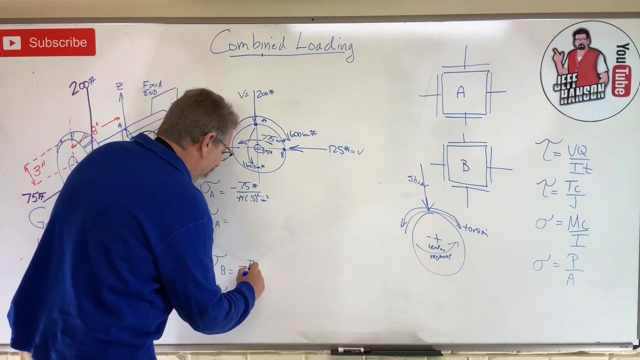 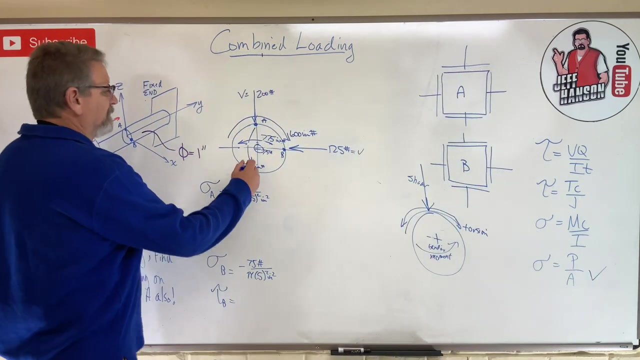 Right there, The area is, the diameter is one. so how about pi R squared Pi times 0.5 squared inches squared right, And B experiencing the same thing: negative 75 pounds divided by pi times 0.5 squared. okay, So that got this guy completely. So we got this one in the middle here. 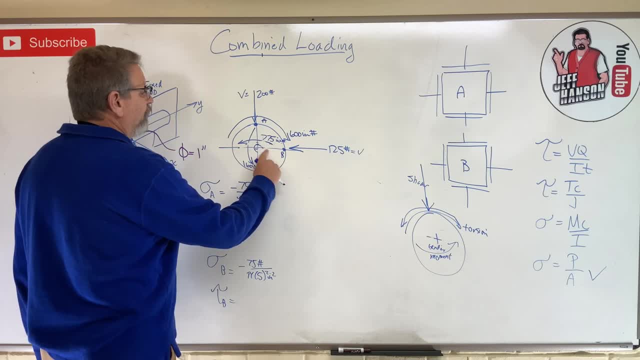 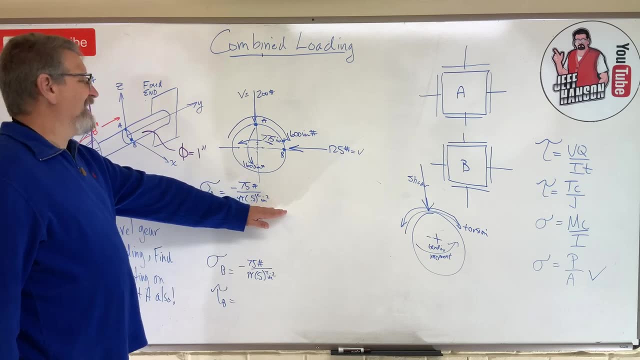 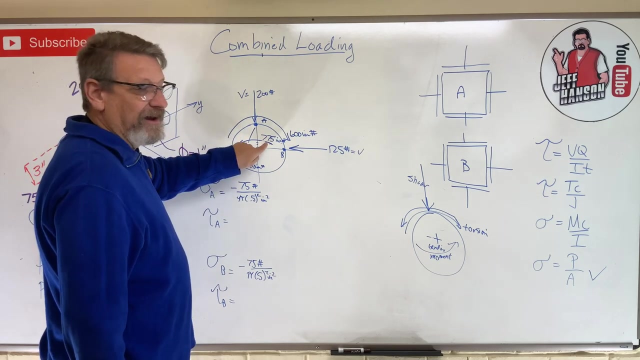 right, We got. this guy is done. I'm going to take him away because he's done. okay, He's done Okay. how about MC over? I stress Okay. now I am point A. okay, The 775 is bending. 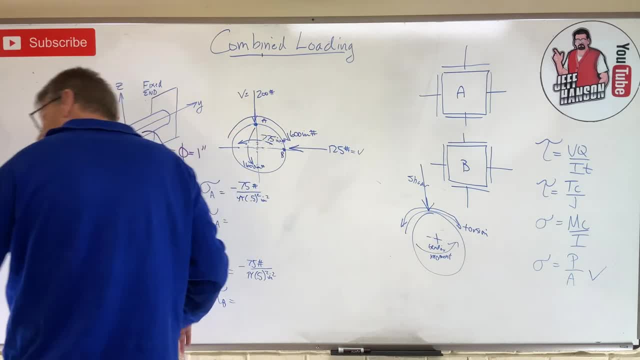 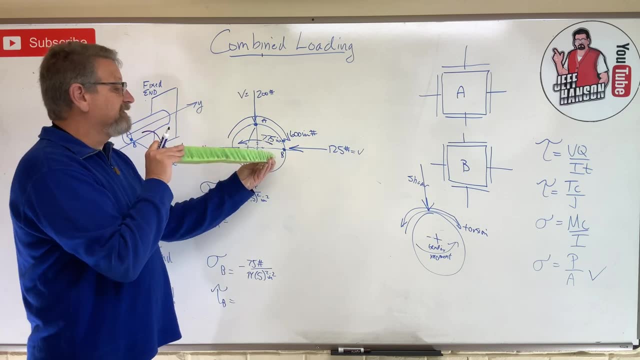 this way. okay, Here's my here. he is right. Point B is on this side over here. The 775 is making me do this number. okay, Oh, point A is on top, isn't it? So if I'm bending this way, where is point A? 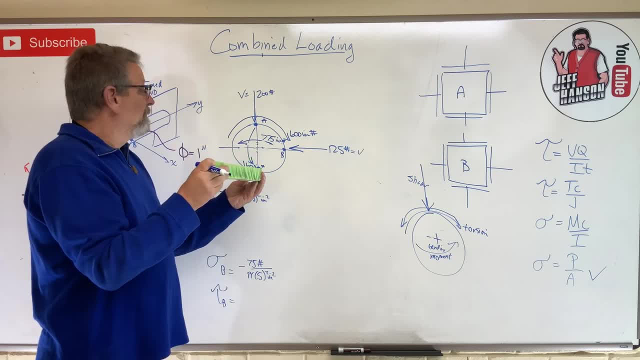 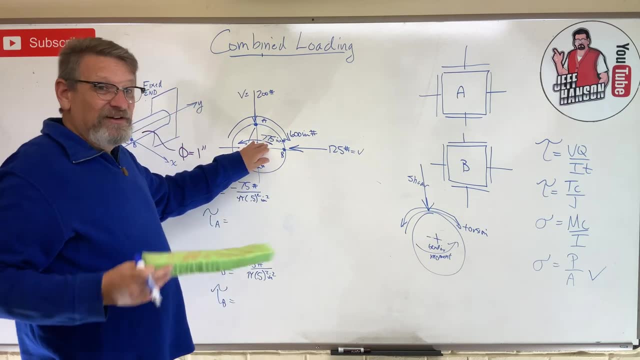 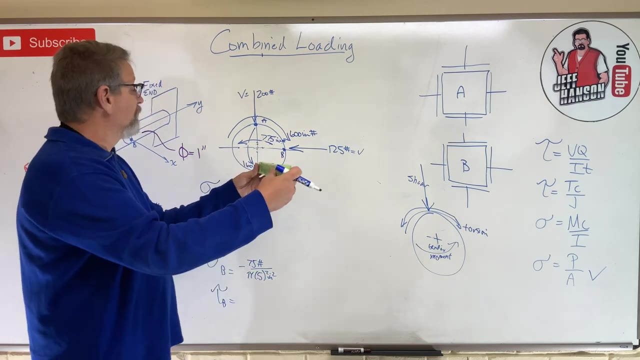 Because this side is in tension, this side is in compression, but Point A is right in the middle. so Point A is what It's on the neutral axis. So the 775 doesn't affect me. point A, Okay. Does the 775 affect point B? Okay, Here we go, 775.. Yeah, Point B is on this side. 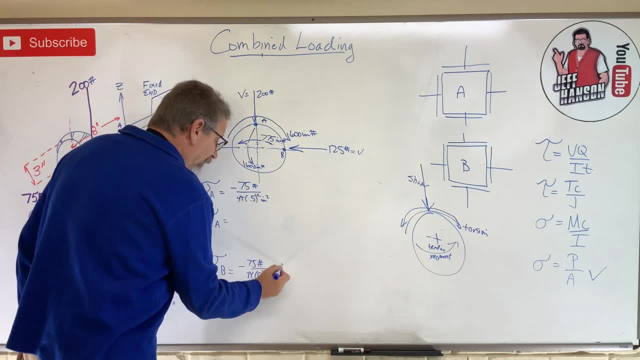 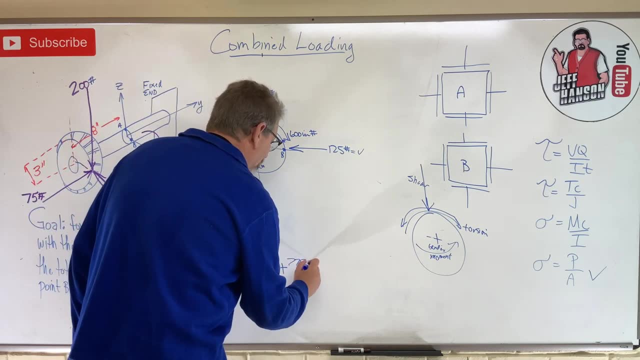 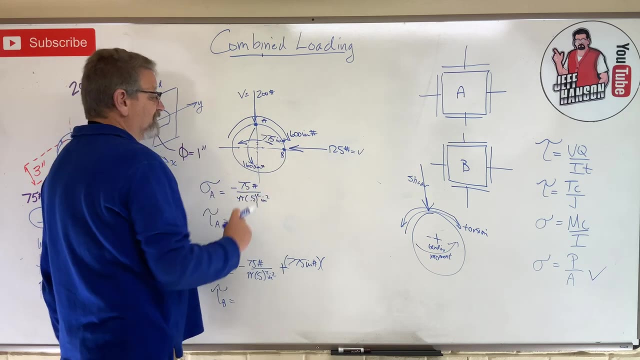 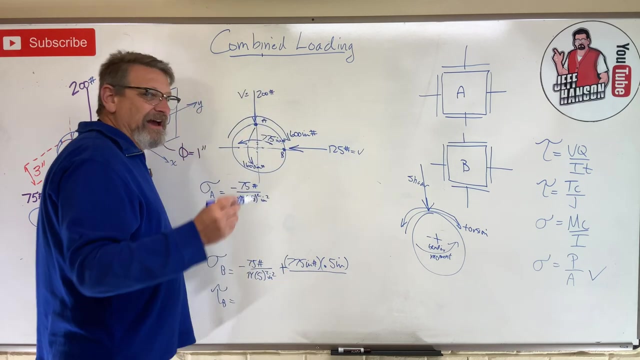 Point B is in tension. So what does that mean? It's a positive. Okay, And so MC over I: 775 inch pounds times C. C is the distance from the neutral axis to the point of interest, And so that's going to be 0.5 inches, Okay, Divided by I. I for a round shaft is what. 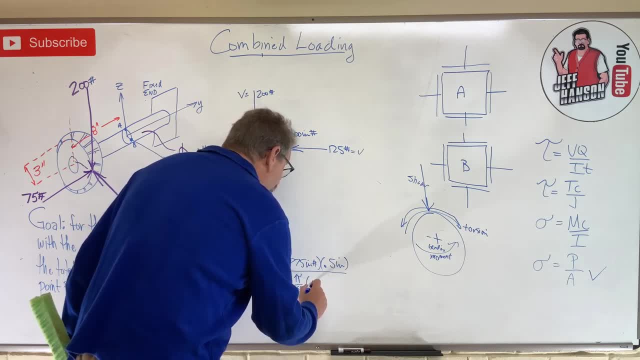 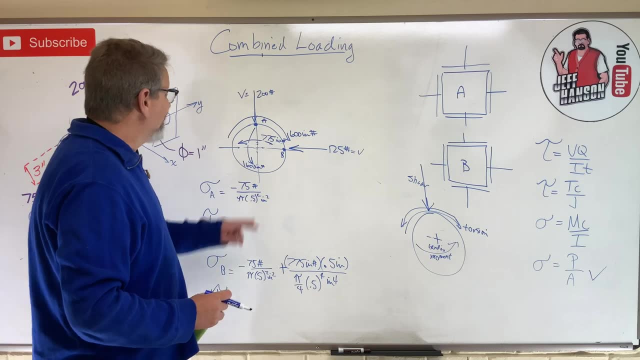 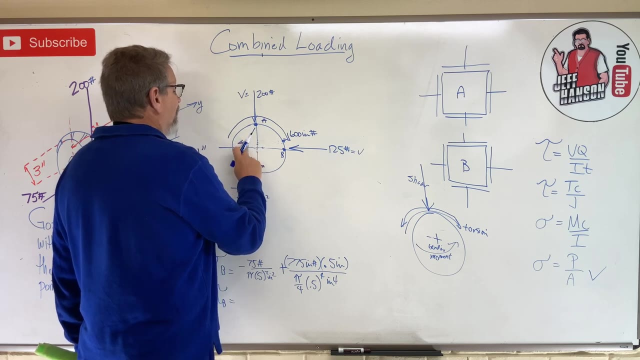 Pi over 4 D, I mean sorry R to the fourth. Okay, And that's got the 775,. right, We took care of you. Okay, We'll get rid of him. It's getting simpler now that stuff is going away, isn't it? 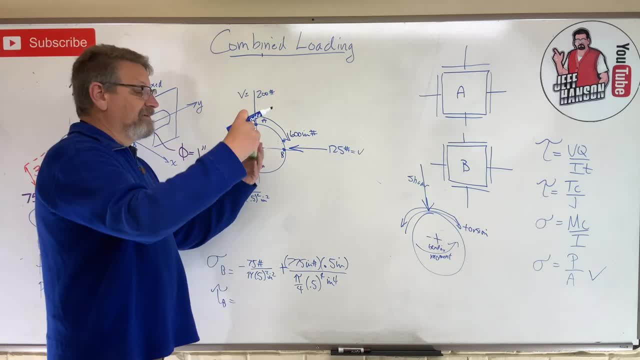 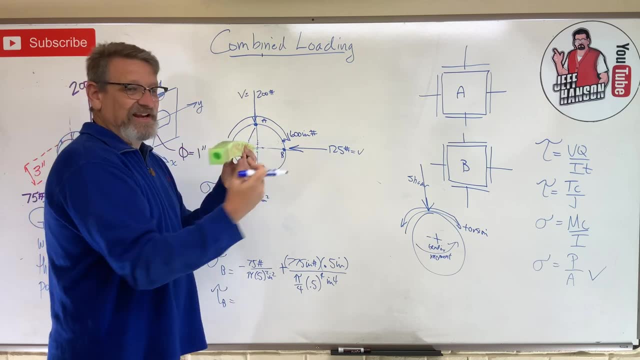 Okay, Now what do we have? We have 1600 bending. The 1600 is bending me down. Okay, Where's point B? Point B is over here on this side in the middle, So point B is on the neutral axis. 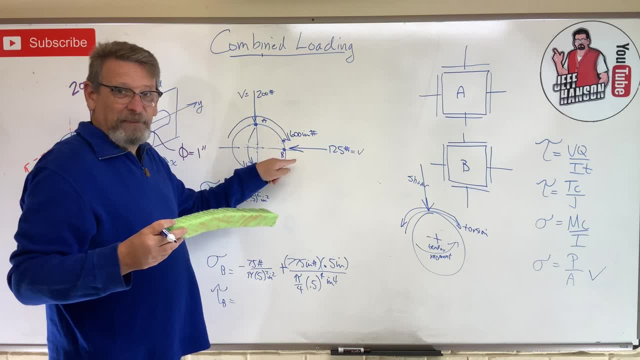 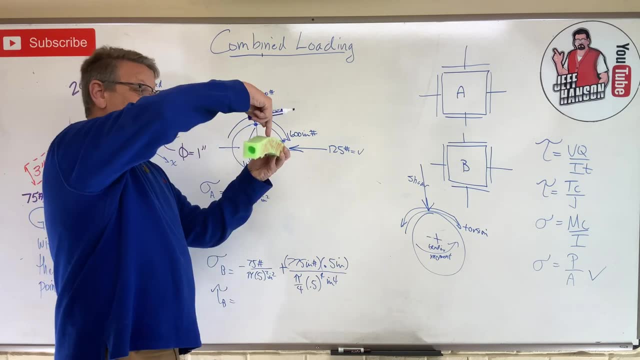 So the 1600 doesn't affect point B, does he? He's on the neutral axis, No stress, Okay, Point A as the 1600, point A is on top. So what's he in Tension, right? 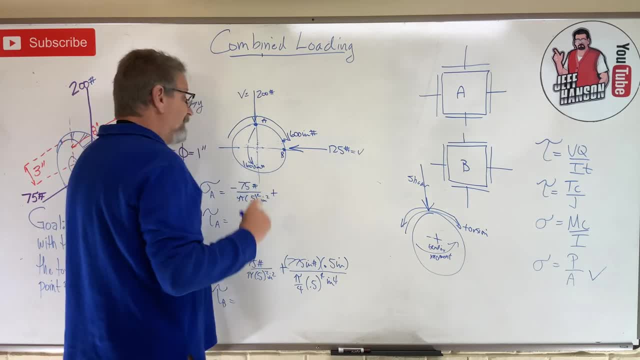 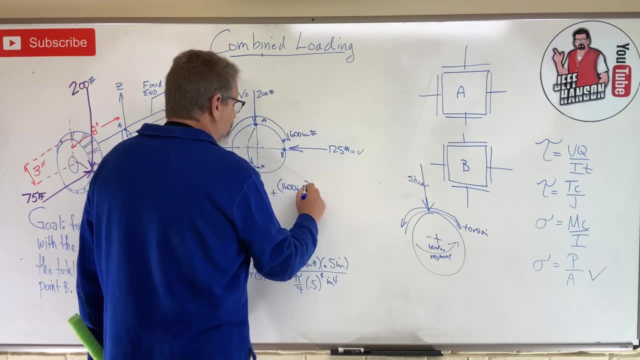 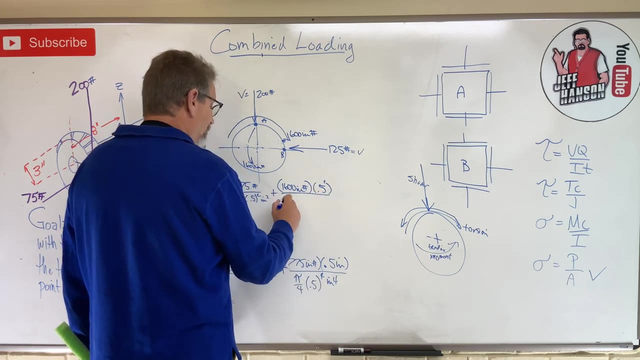 So we're going to have a positive for tension, Okay, And we're going to have MC over I. Here we go. M is 1600 inch pounds, Okay. Times C: again 0.5 inches Divided by I, which is the same I down. 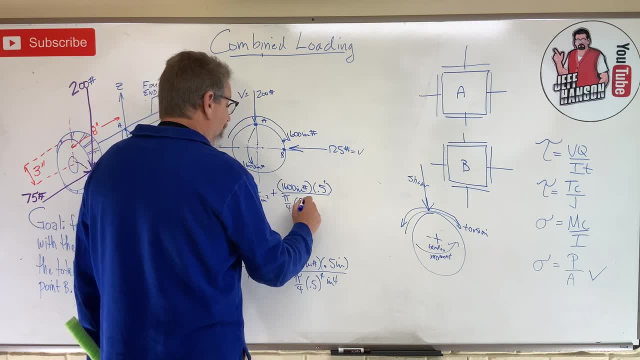 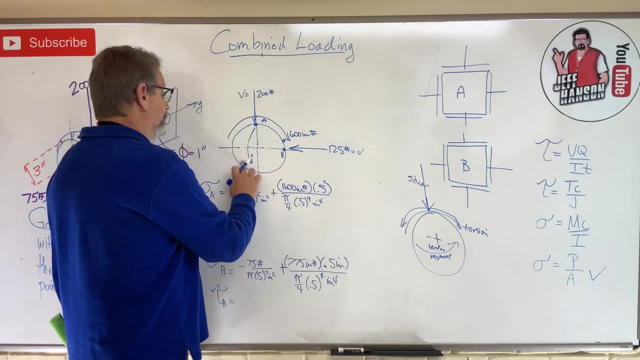 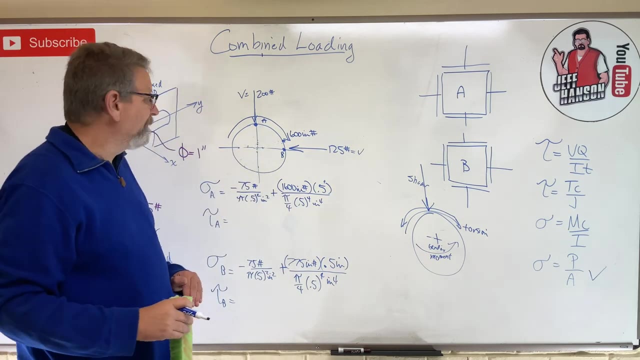 there. pi over 4 times 0.5 to the fourth, inches to the fourth, And that's got my 1600 taken care of. Okay, So we took care of all of the sigma stress in both A and B. All right, Now we're on to tau stress. 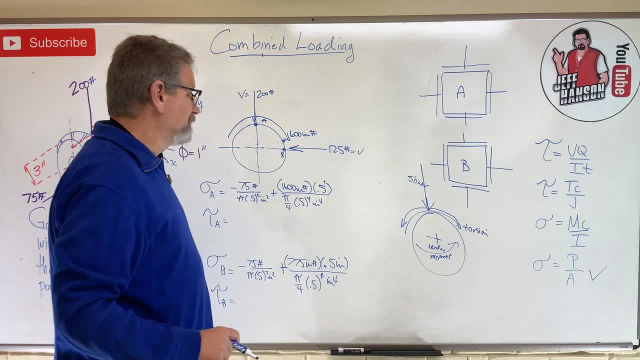 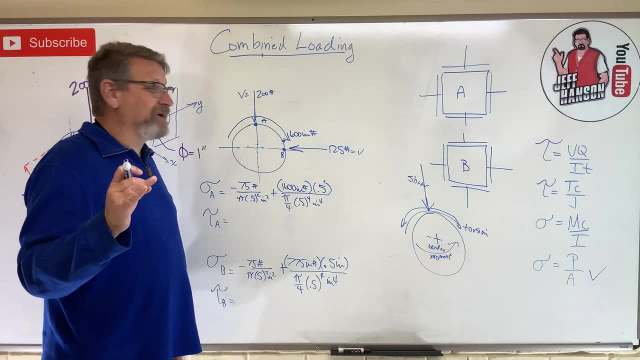 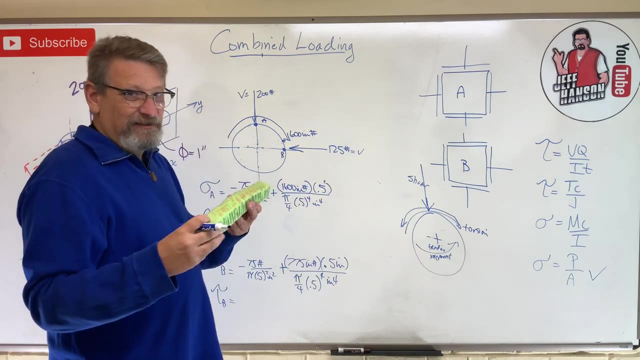 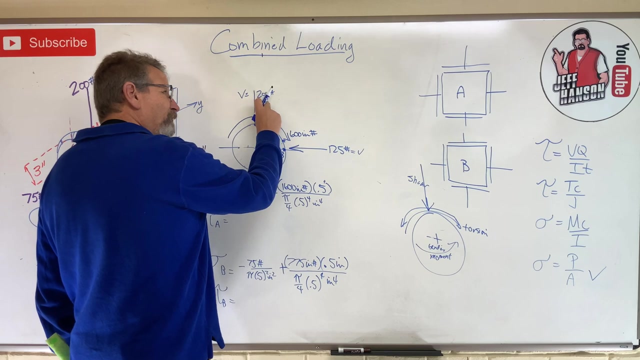 Okay, What VQ over IT? Oh boy, All right, I'm at point A. Okay, Now remember when you're figuring VQ over IT. okay, the neutral axis- the bending neutral axis right, is always perpendicular to the V force. So when I'm calculating the V force from the 200,. 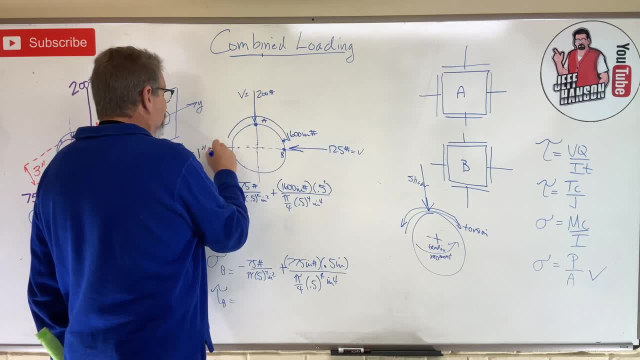 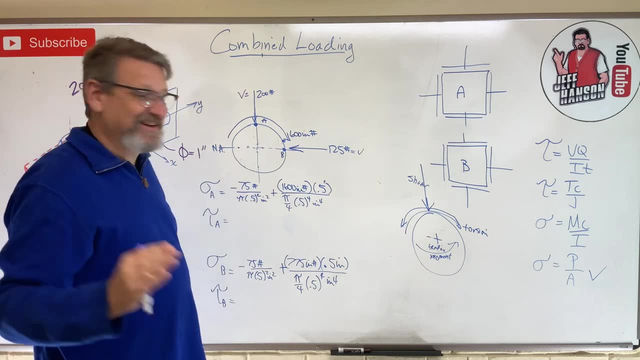 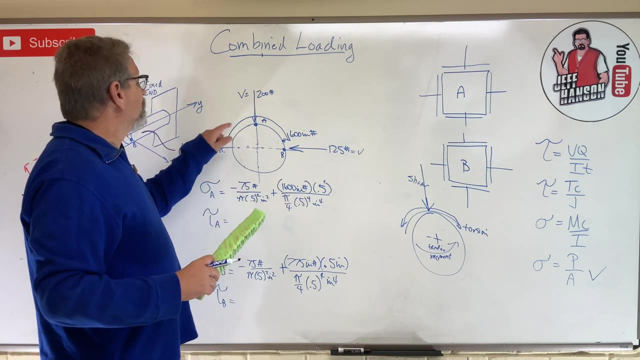 I'm talking about a neutral axis. that's here. Okay, When I do the 125, the neutral axis is this way, It's always perpendicular. Okay, So let's talk about the 200. Okay, Well, if I am calculating VQ over IT, okay for a shear. this direction, which means my neutral axis is 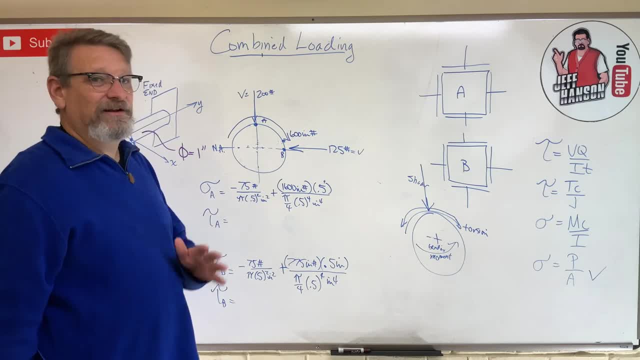 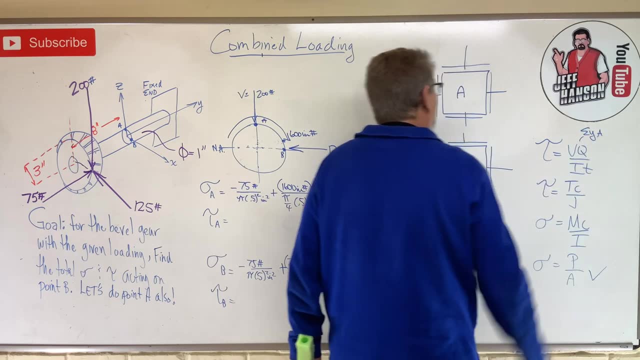 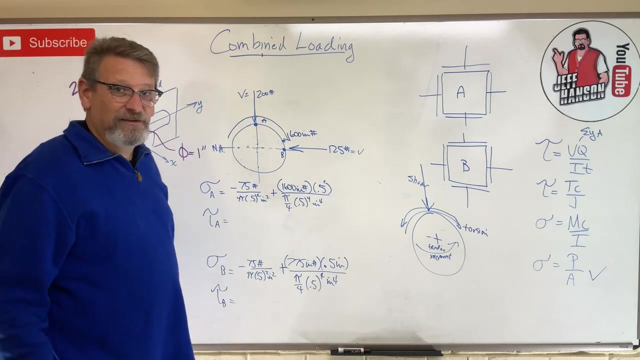 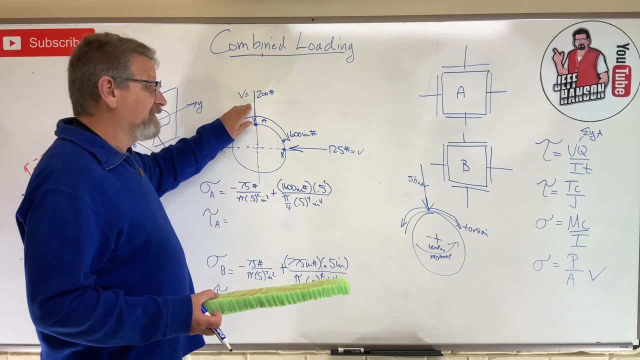 horizontal. Okay, How do I calculate Q? Do you remember how to calculate Q? What is Q? The sum of the Y times A, right Above or below the point of interest. So how much area is above point A? None. What does that mean? That Q is zero for the 200, which means the 200 doesn't cause any. 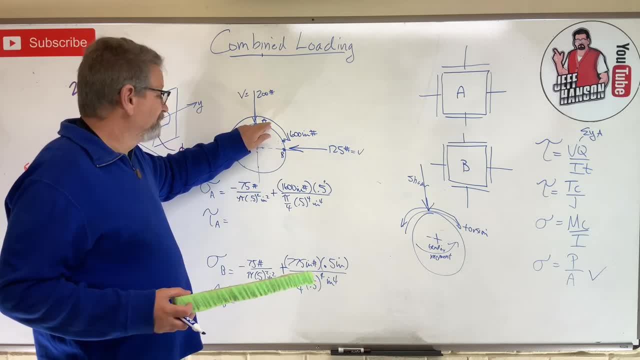 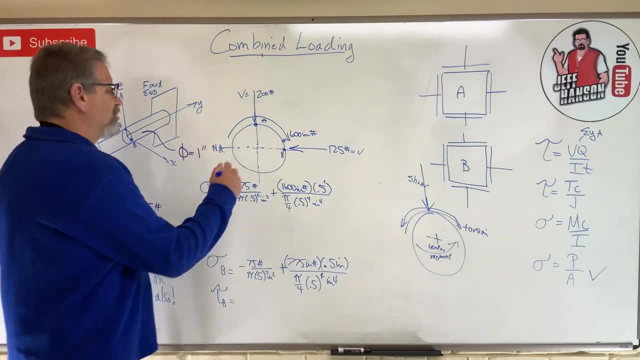 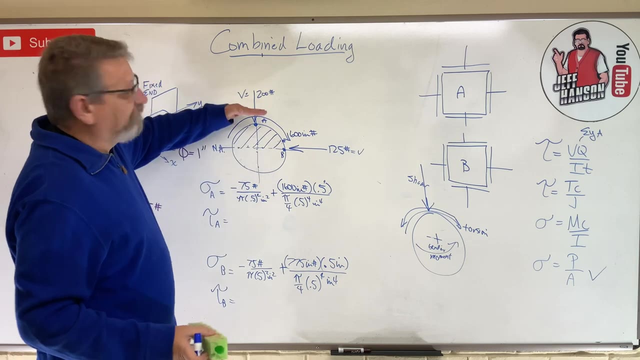 shear whatsoever at point A. Okay, The 200 doesn't. does he do anything for point B? Well, yeah, he does, right, Because what is Q for point B? Q for point B is this. It's all of that area above point B, isn't it Okay? 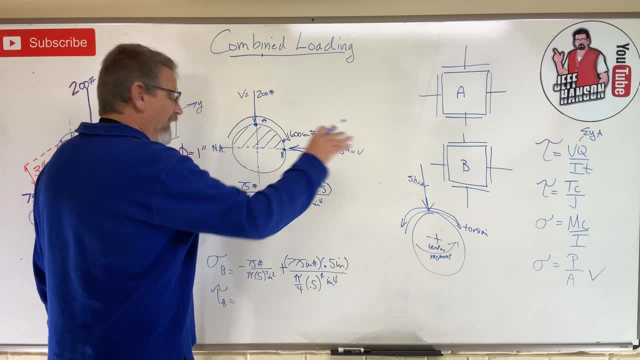 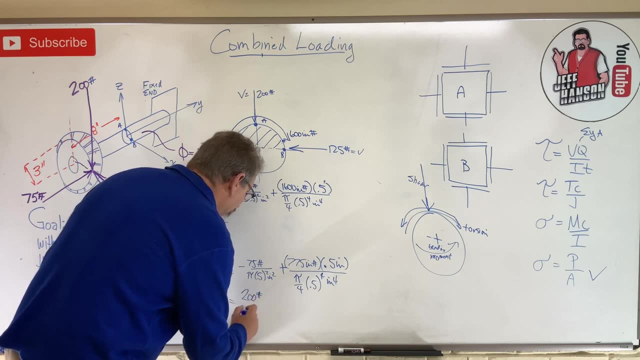 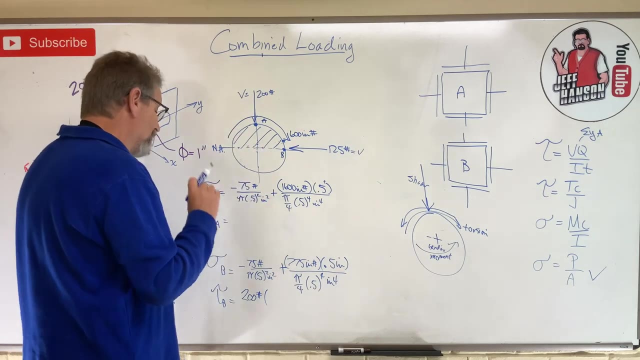 So let's do this, Let's write down tau for point B and it would be this: VQ over IT. So V is 200.. Okay, Q, whoa, Q is that shaded area. So it's Y times A. Okay, So the area is pi R squared, pi R squared. 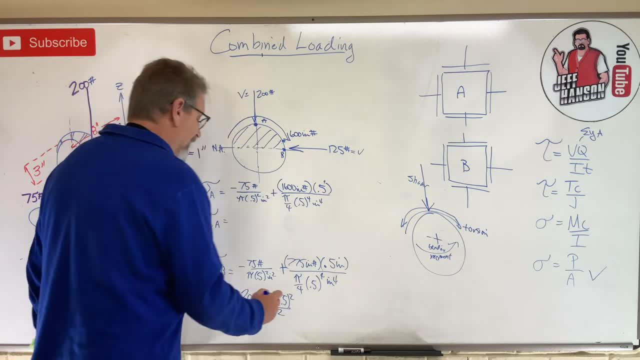 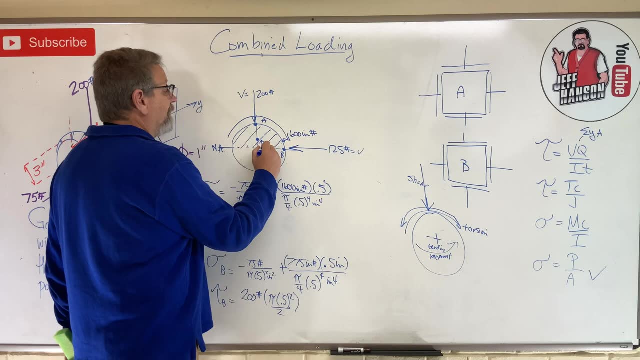 divided by two, isn't it Right? Because it's a half a circle times Y bar. So where is Y bar right of that area? Where is Y bar of that area? Hey, that's half a circle. I remember that from. 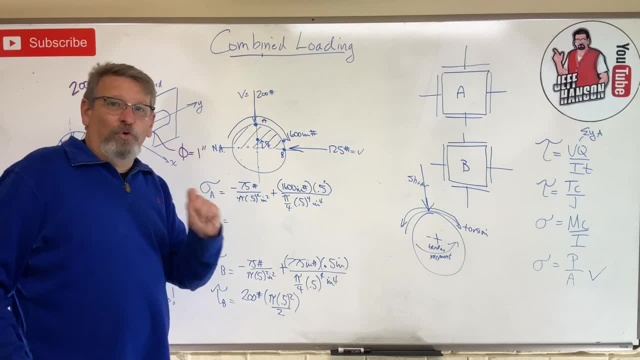 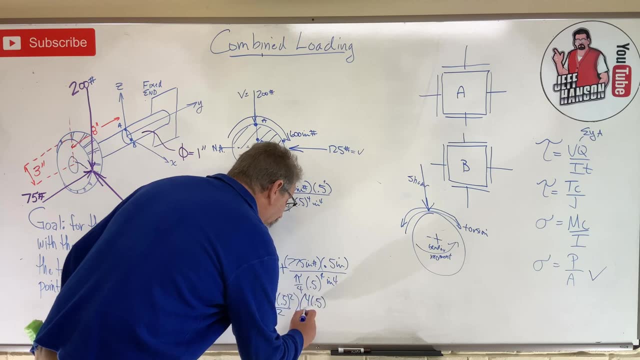 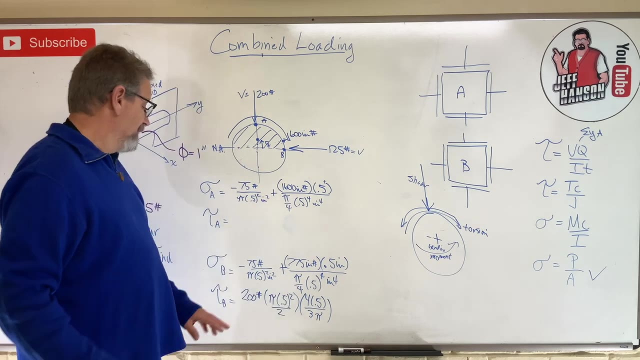 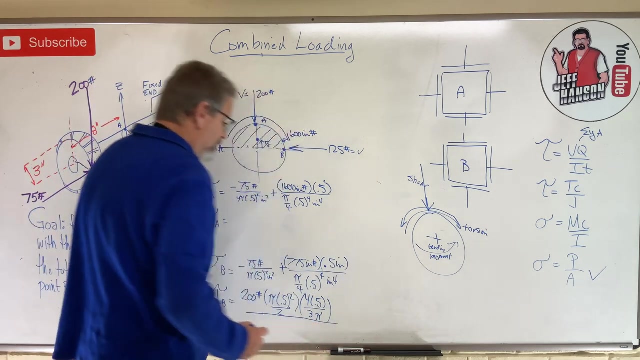 my centroid table. It's 4R over 3 pi, isn't it? So times 4R.5 over 3 pi. Okay, So this is Y bar. that's A right. So this is VQ divided by: divided by what IT I we got I everywhere, don't we? There's I, right there. 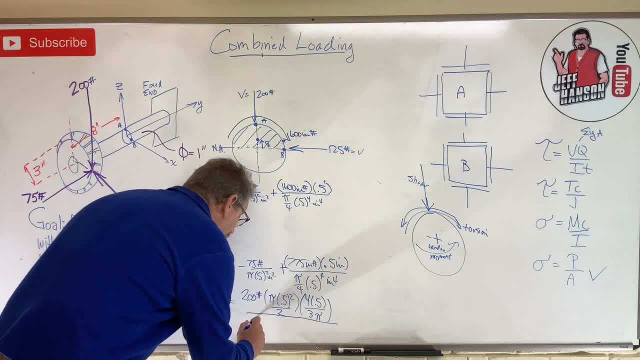 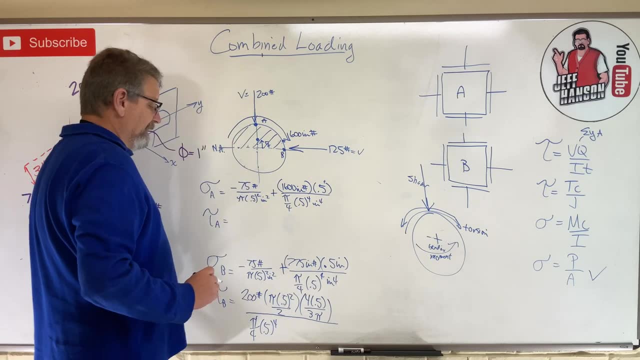 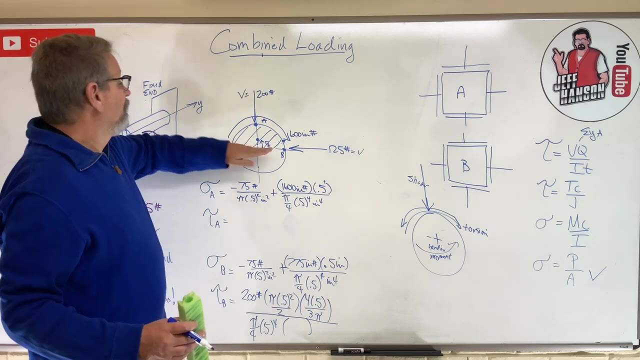 No, there's I right there. Pi over 4 times 0.5 to the fourth. Okay, That's I times T, What's T? What's the thickness? How much beam do I have to tear away? Well, I have to tear away that thickness. right there, The thickness. 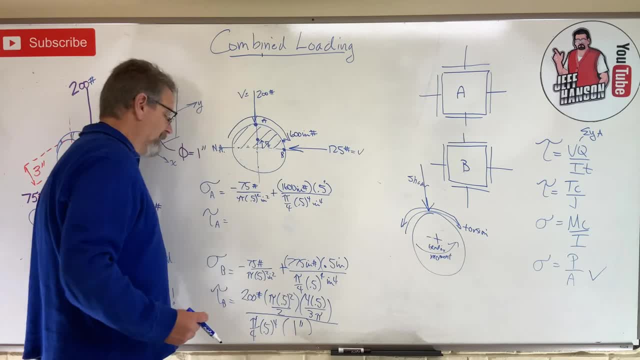 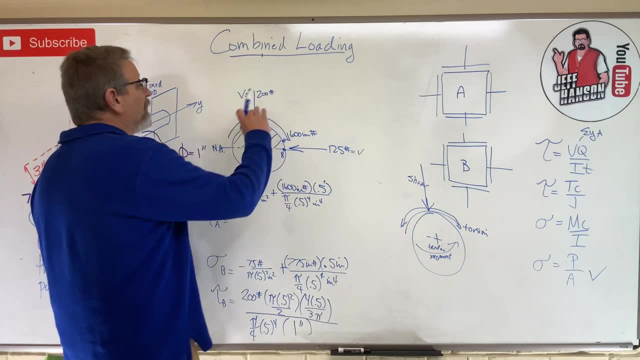 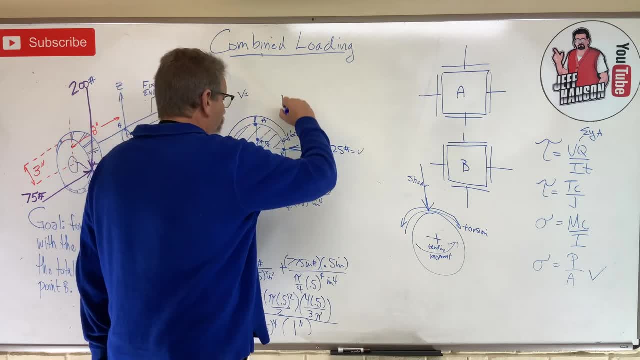 200 over here. So I'm going to move this 200 over here, Just like this. Look what I'm going to do. I'm going to move him over here. Boom, There he is. He's still pressing down, but 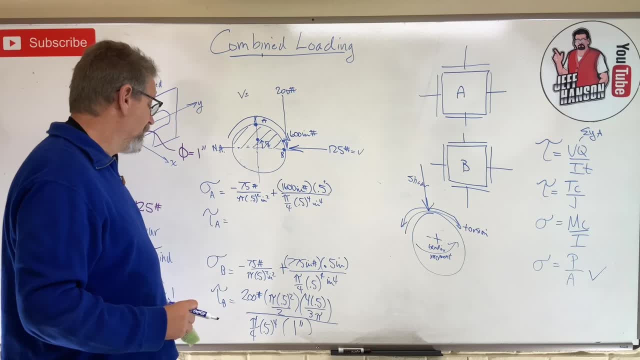 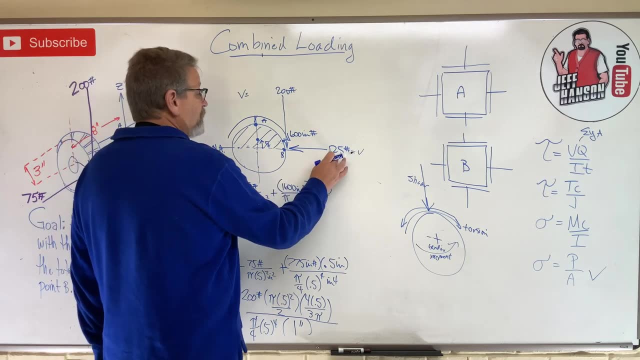 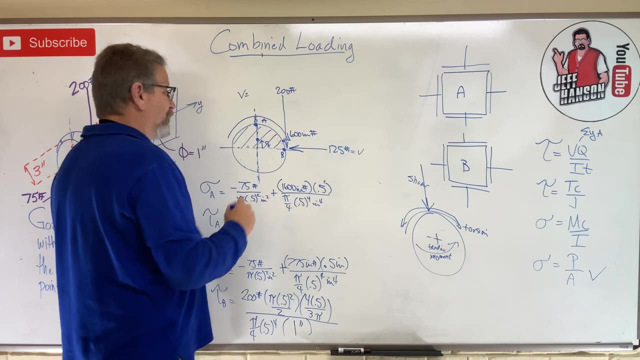 I just moved him over so I can see him pressing on point B. Okay Now, same exact steps, But now let's talk about the 125.. Okay So, now my neutral axis is horizontal. Okay So, this is my neutral axis for the 125. 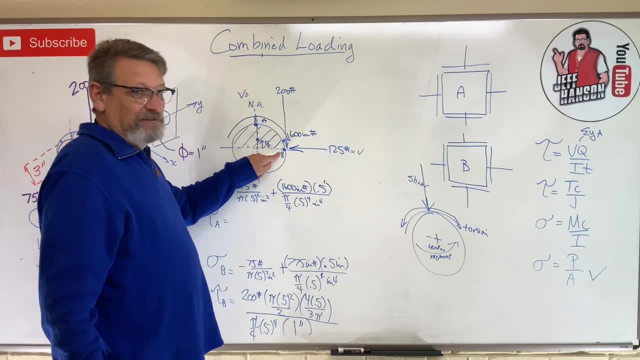 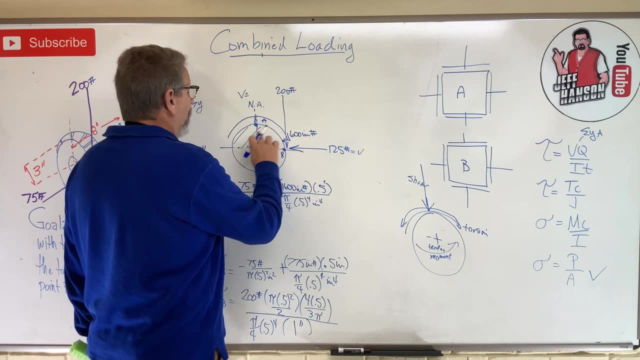 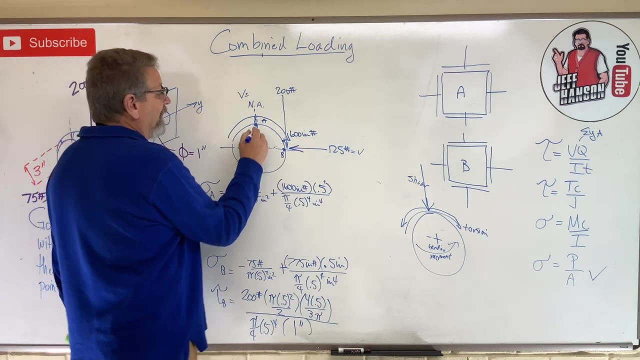 Does the 125 make shear at point B? How much area is above point B? How much? Well, a grand total of zero. okay, So now we move over to point A. How much area is above point A? Well, it's this area here, right? So it's just like we did before, down here. 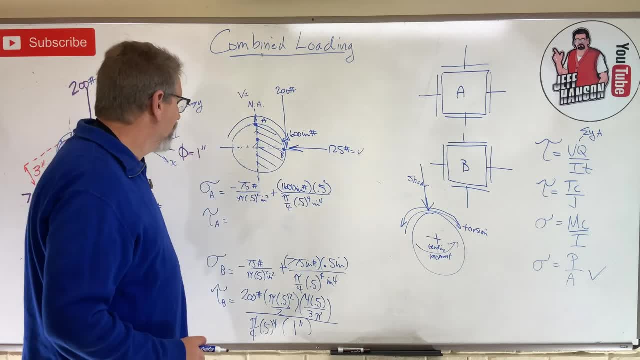 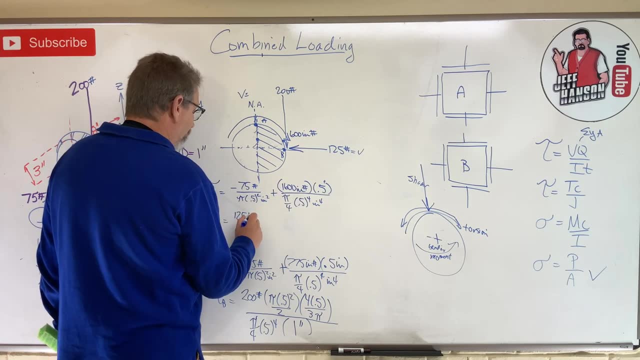 but a different direction. okay, So this is about point A. So it's VQ over ITV 125 Q. okay, Same thing as it was down here: pi times 0.5 squared, divided by 2 times that guy Y bar. 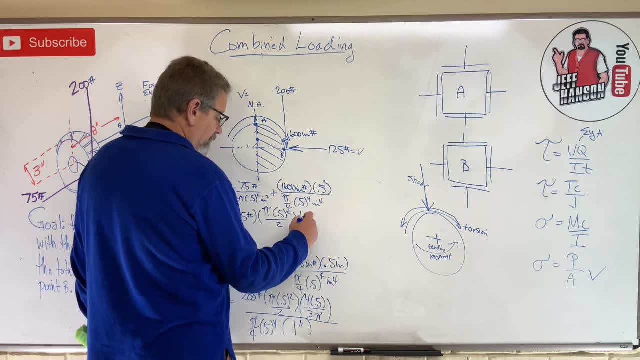 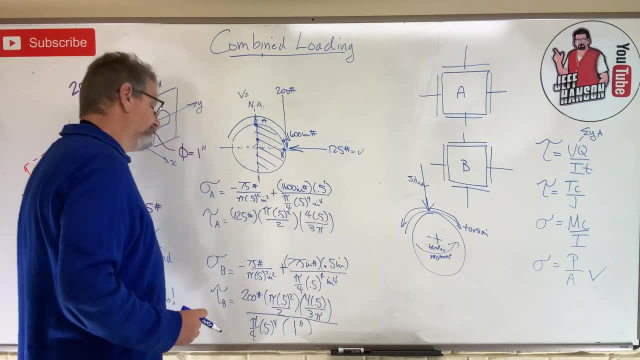 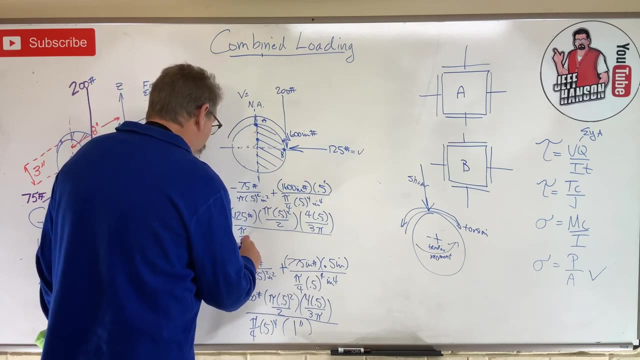 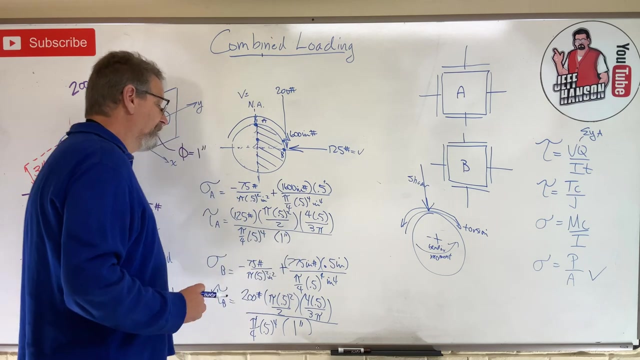 right, Which is 4R, 4R over 3 pi- okay. Divided by IT, pi over 4, times 0.5 to the 4th times 1, okay, And so that's the 125.. And the 125 doesn't affect point B, but he affects point A. I'm 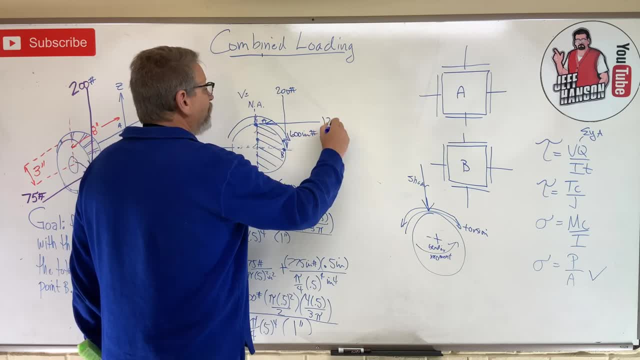 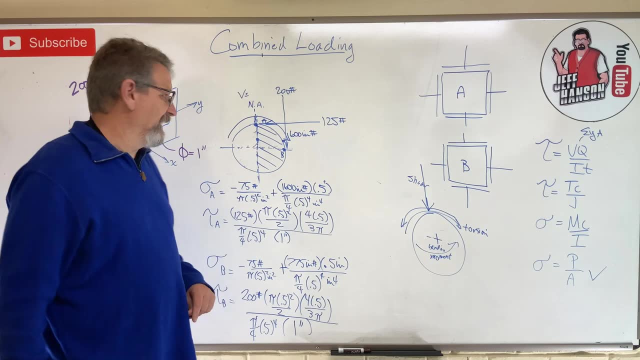 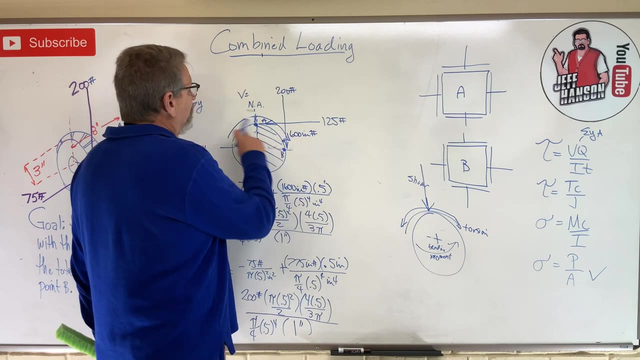 just going to move him over here like this: okay, 125.. Okay, Because now what? Well, now it's torsion time, okay. So what I'd like to do is this: If I am at, if I have torque, this way, right When that torque comes around to point B. 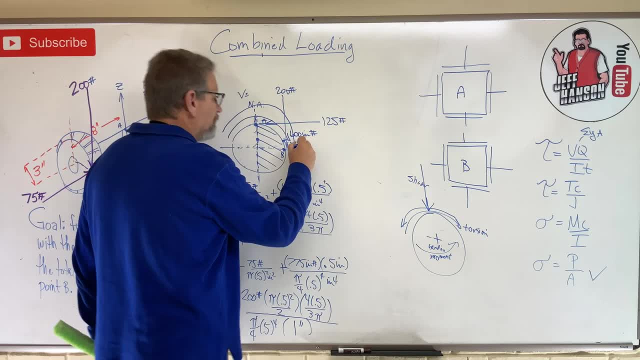 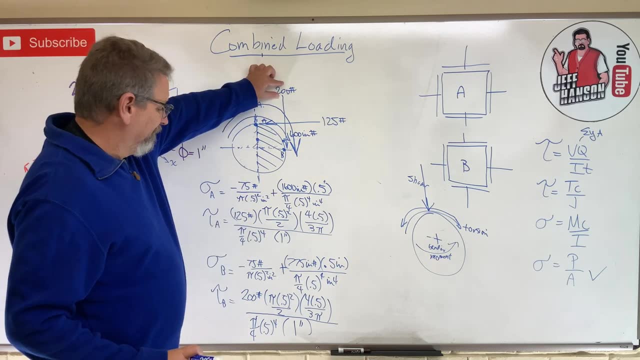 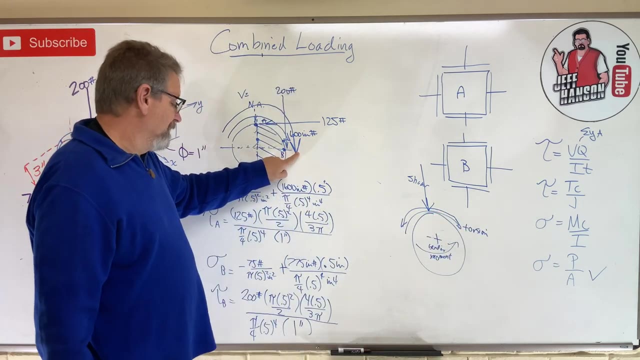 okay. What's it doing at point B? It's pushing down, isn't it? So what I'm going to do is this: tau that I figured down there is going to add to this TC over J. tau, that's also going down at point B. okay. 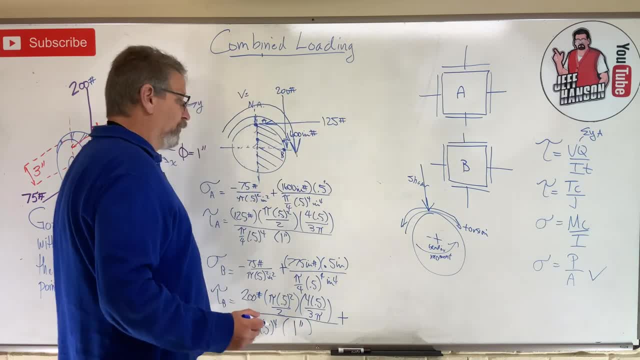 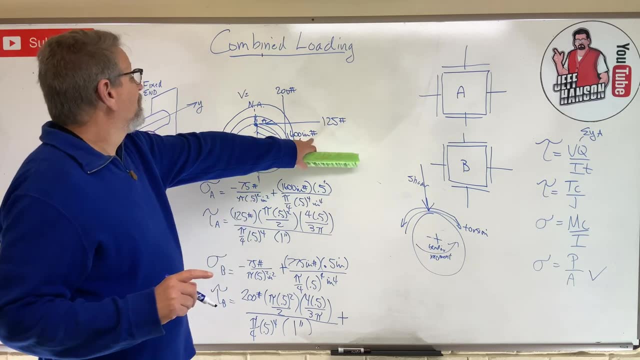 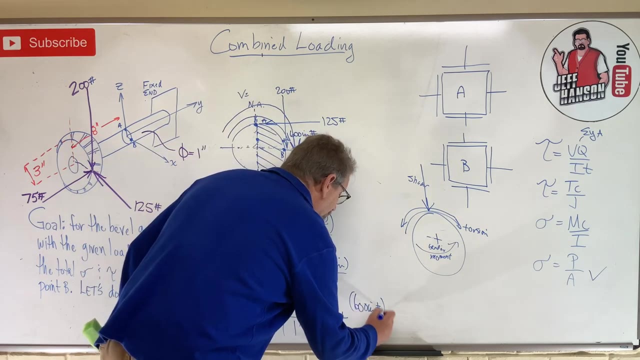 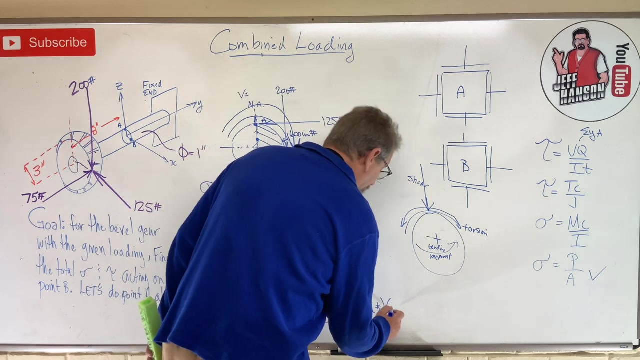 So I'm going to have this additional shear force over here, shear stress, rather okay. So TC over J. T is what? 600 inch pounds? 600 inch pounds times C, What's that? What's the distance from the neutral axis to the point of interest? 0.5.. And J, What's? 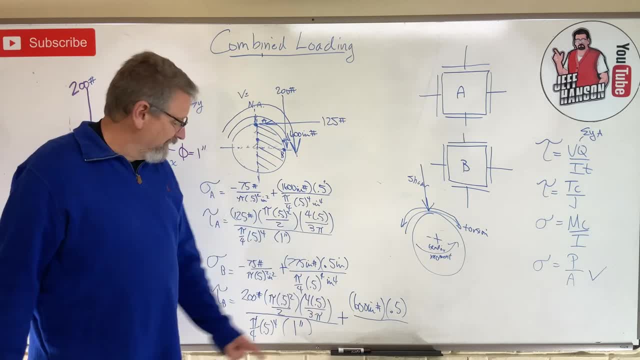 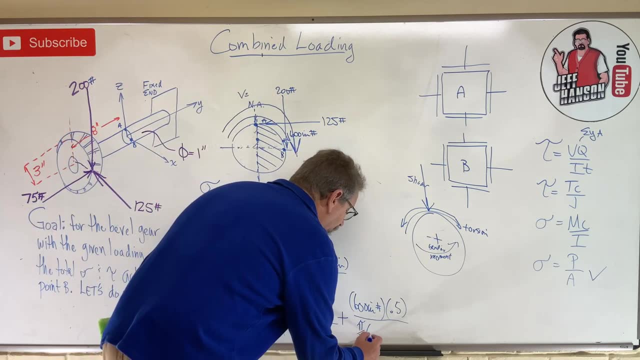 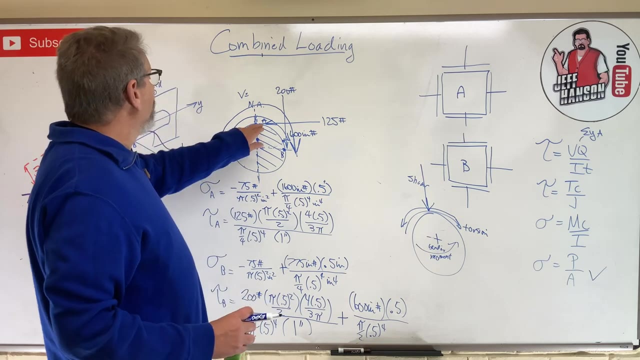 the difference in this I and J. that goes over there. Instead of pi over 4,, J is pi over 2.. R to the 4th, 0.5 to the 4th. okay, Now let's talk about point A, right As that torque comes. 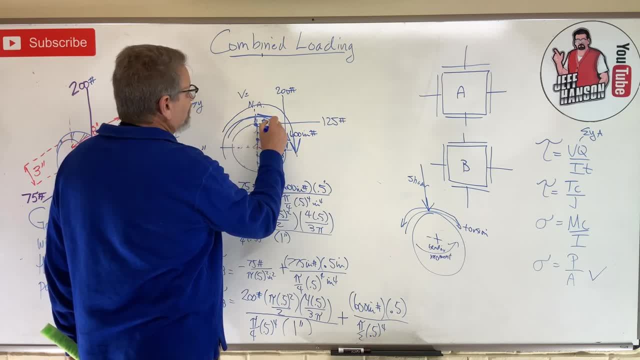 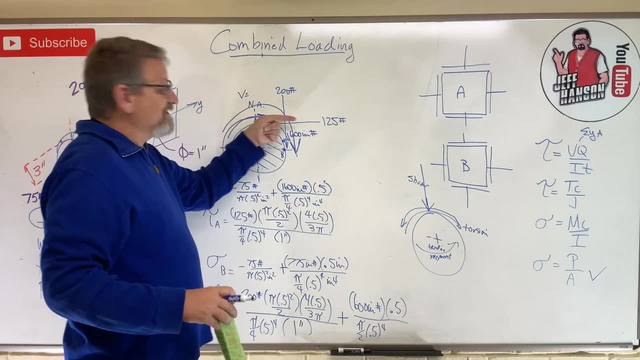 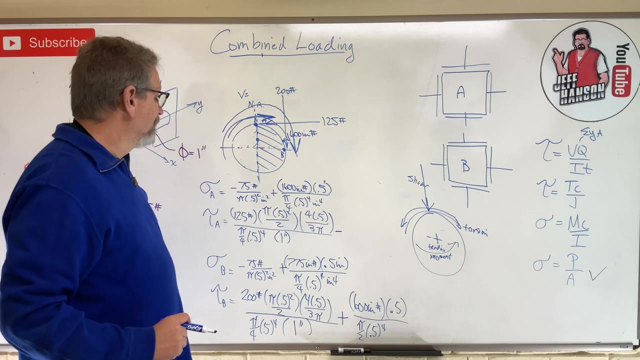 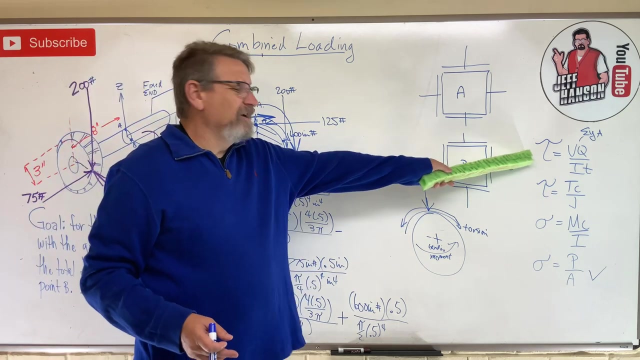 around to point A. which way is he pointed? Well, the 125 went that way, but the torque here is working against the 125. So he is actually going to subtract, subtract, right, And don't worry about the signs on this right now. Just always consider this guy here, the VQ over IT always. 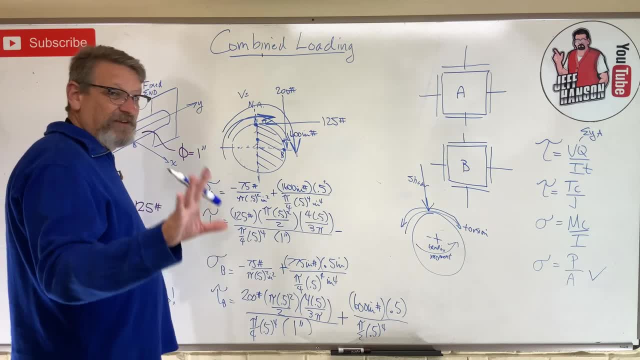 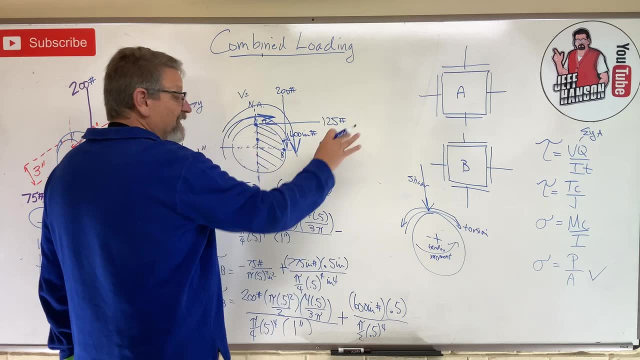 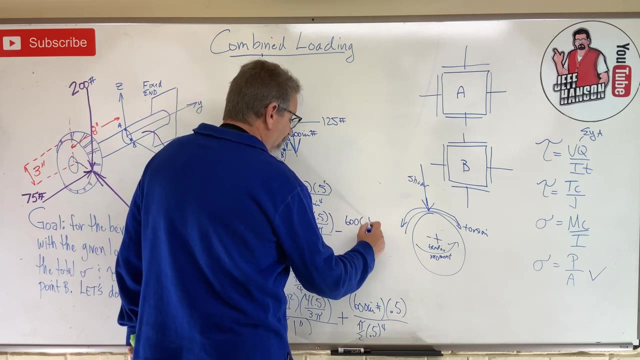 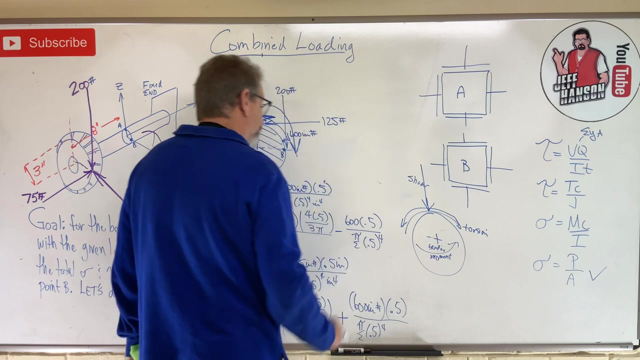 consider him positive when calculating this And I'll show you how to fix the sign here in just a second. Okay, So this guy here, the 600 is working against the 125, so minus, But the same number, isn't it? 600 times 0.5 times pi, over 2 times 0.5 to the 4th. okay, Same number. So that's it. 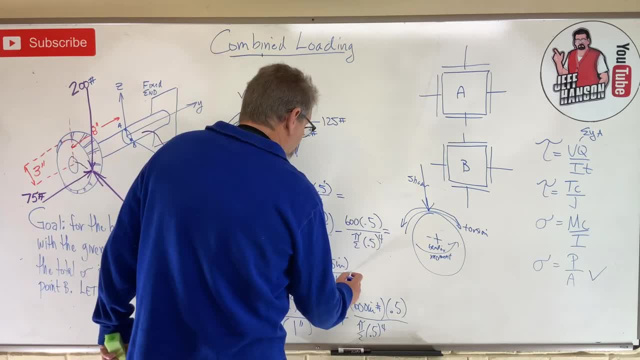 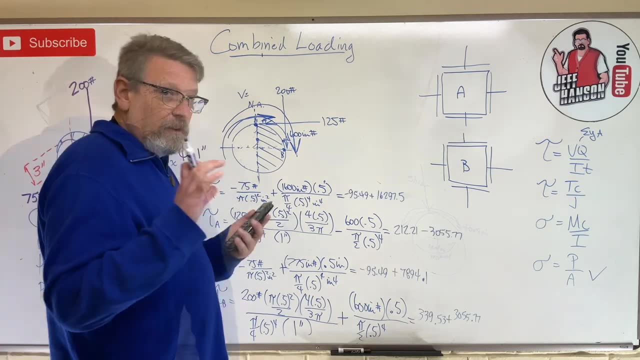 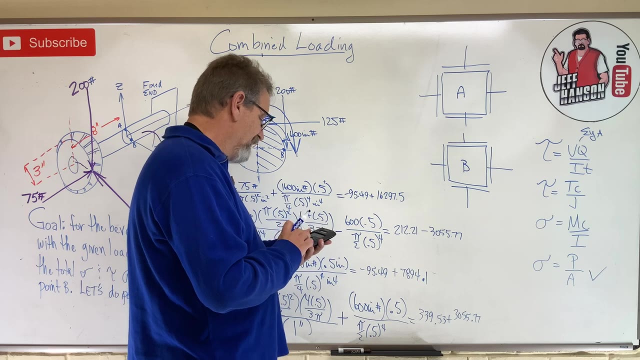 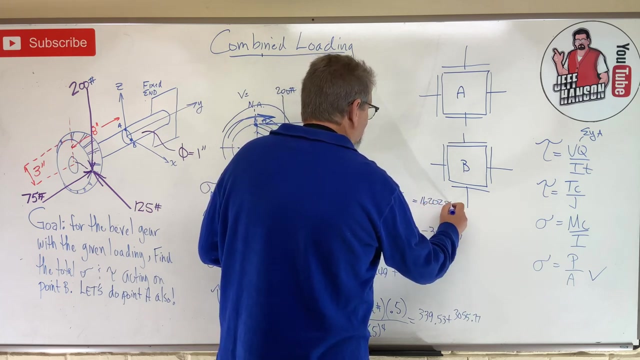 So now I need an equals, an equals, an equals and an equals. okay, Let me calculate that and I'll tell you what those equal. Okay, so I've like got all this added up here. So here we are going to final calculation: 16297.5 minus 95.5 is 16202.. And that's PSI, okay, 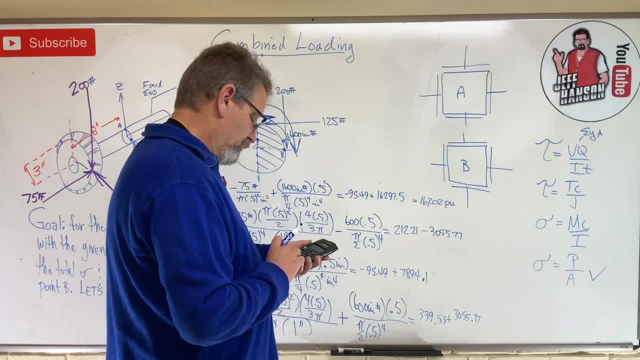 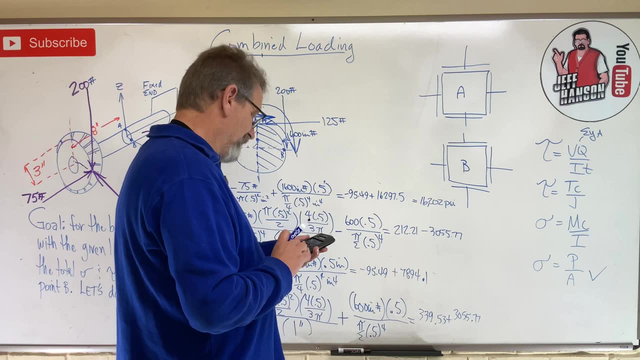 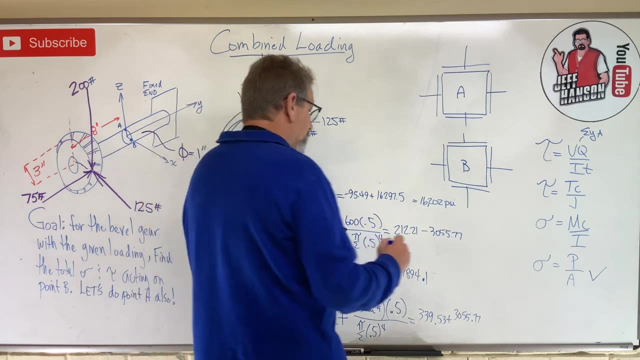 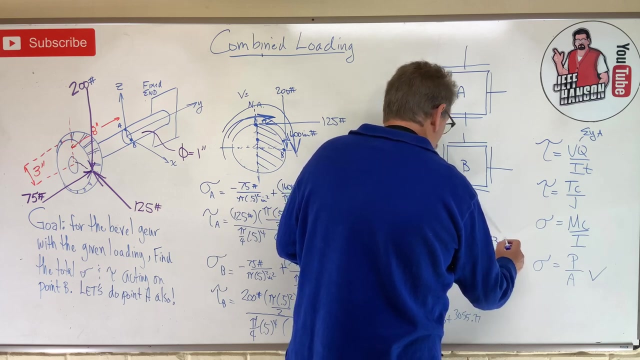 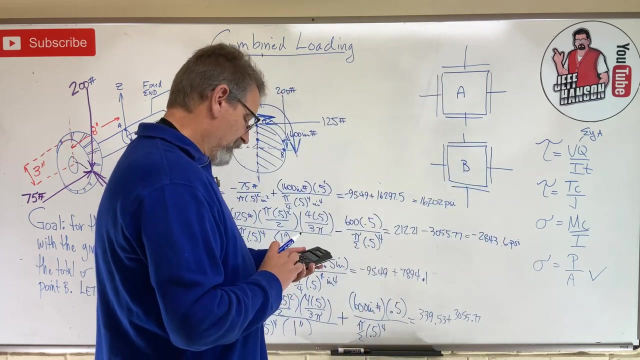 And the next one down here: 212.21 minus 3055.77 is going to be 28,. it's negative 2843.6,. okay, Again, PSI, Okay. and then the next one: 7894.. 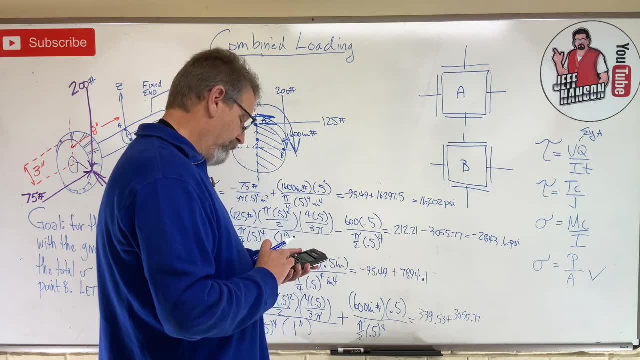 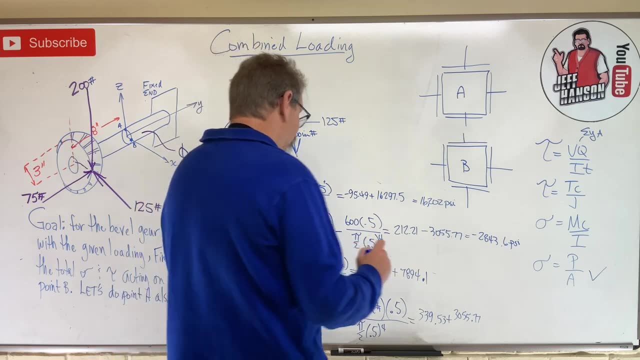 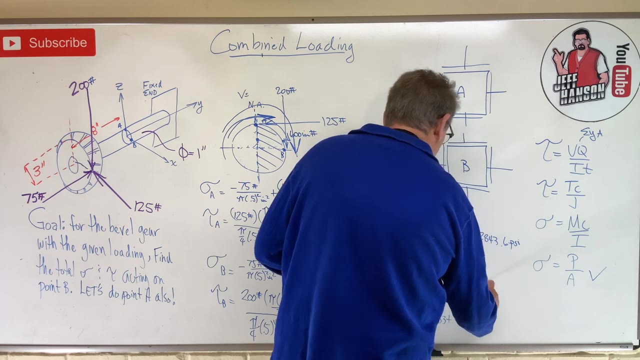 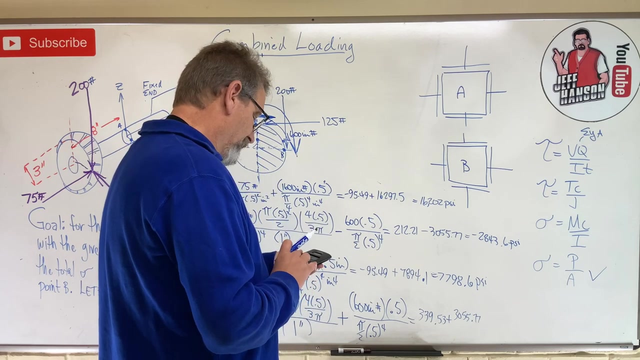 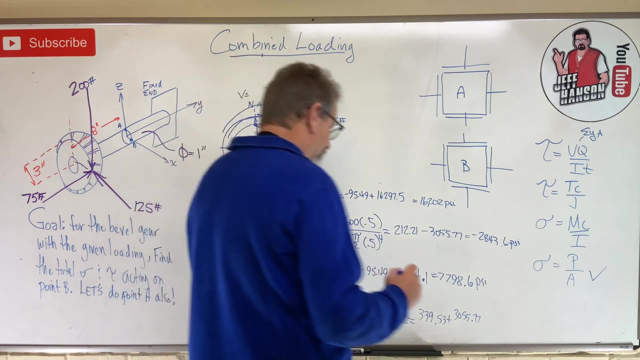 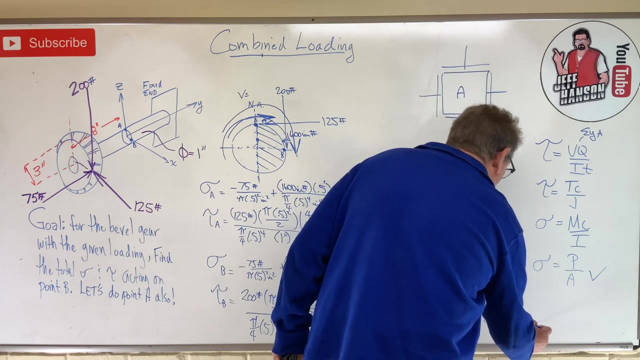 0.1 minus 95.49 equals 7798, 0.6 PSI. And last one: 339.53 plus 3055.77 equals 3395.3.. Okay, PSI, Okay, Are you with me Holy? 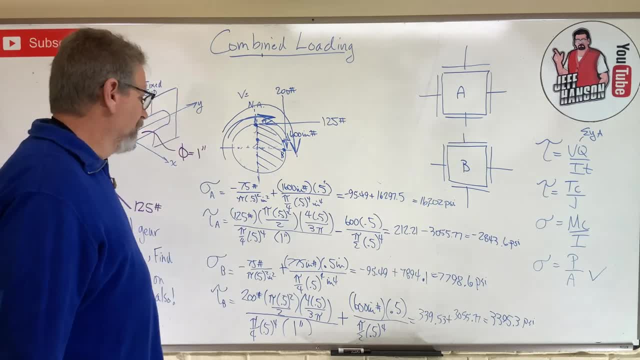 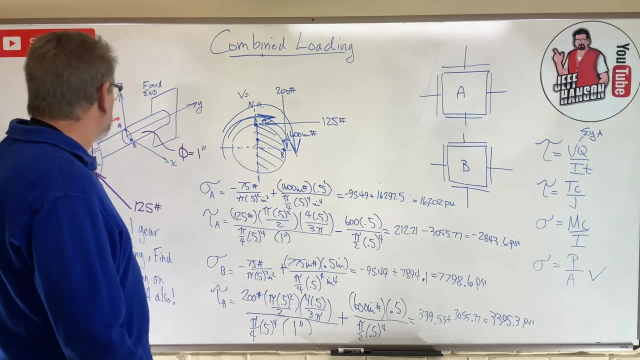 kalabunga dude, Here we go. Let's see if we can figure out our directions now. okay, Last step, Number one. I'm only going to have, right on point A, a computer that does all these general equations. 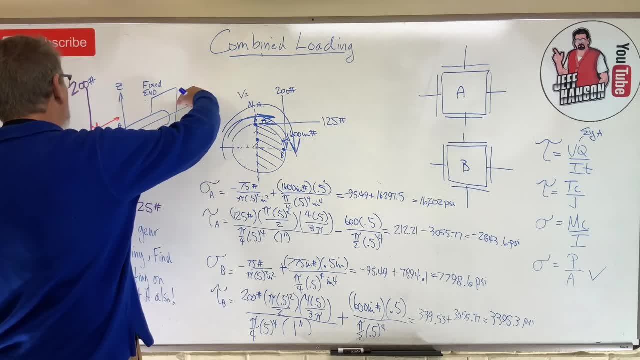 I guess they should start studying them right away. but first we need to do those fractions. Number one, we need to expect the result until the correct answer is given. Okay, 53034.825.ž. Final estimate. Now, at least one is equal. So this number- and I don't want to exaggerate- I'm going to say this. so I'm going to say this again, and we always do It's difficulties. don't become boredage, Let's do this. We just choose to help you out Because, again, it's all genius when you do that and if they boxes and we estimate that you 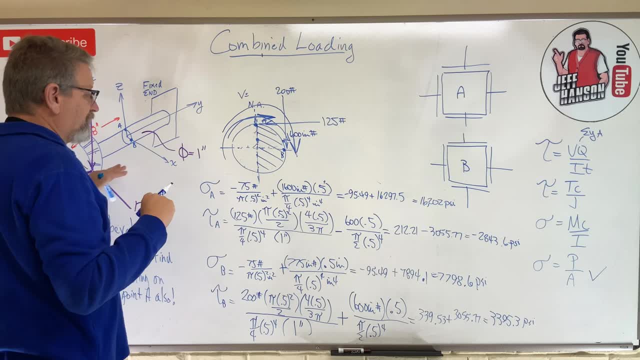 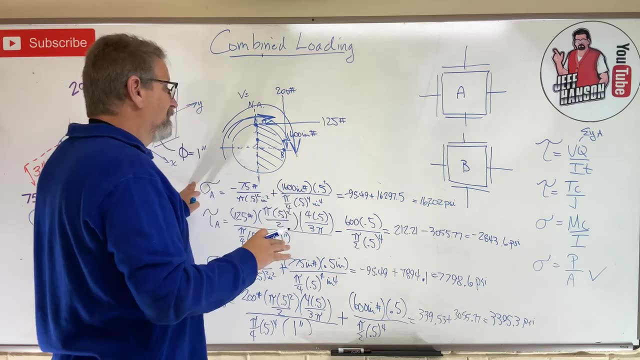 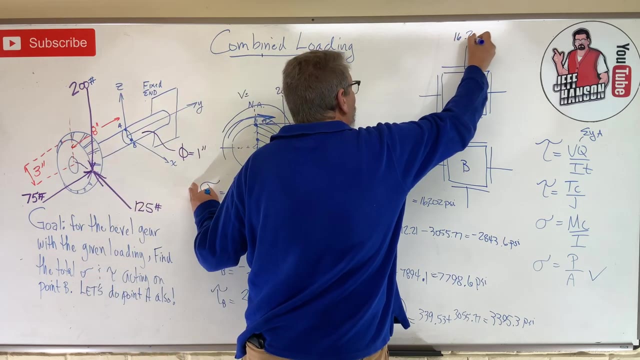 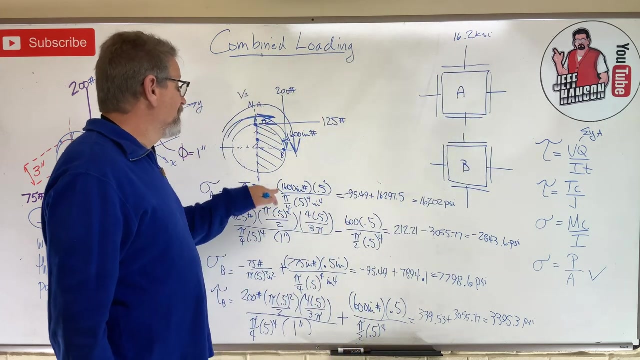 a compression in the y direction. so i'm only going to have a compression in one direction, right, i'm not going to have anything in the x direction. so on my a i'm going to have a sigma stress of 16.2 ksi. okay, and we said what well, this was into a compression. but that guy was in tension and 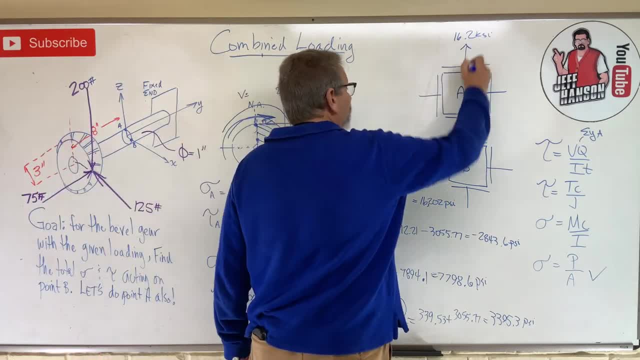 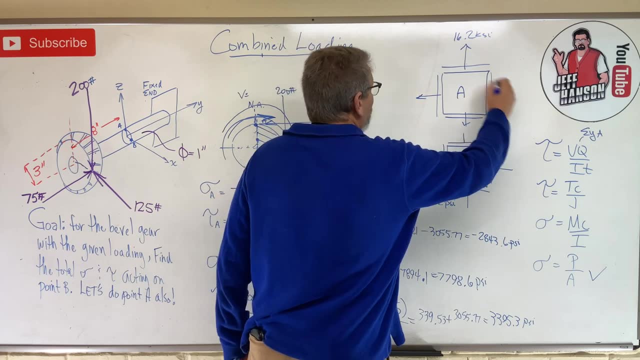 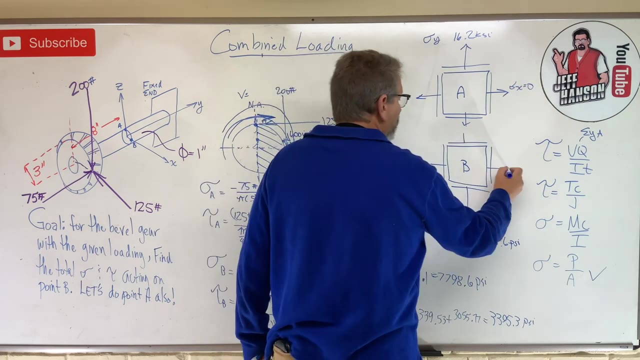 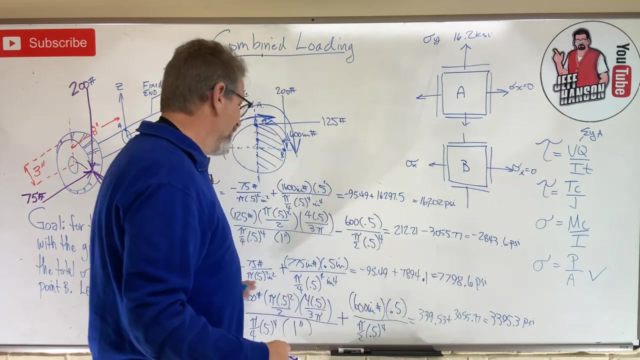 guess who won out? it's intention, isn't it? because i got a positive value over there, right, and then this guy over here, right. this is sigma y. sigma x equals to zero. same for this guy. sigma x equals to zero, sigma y. what do we get? we got a positive value again, so intention. 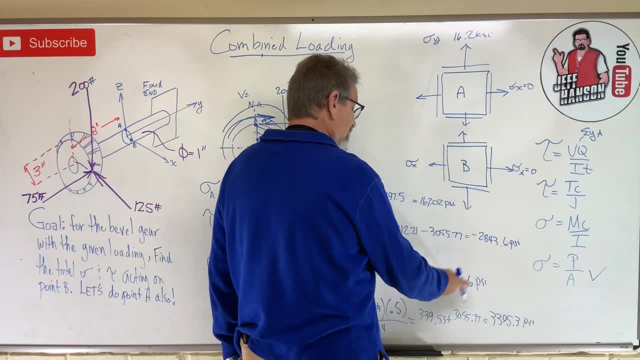 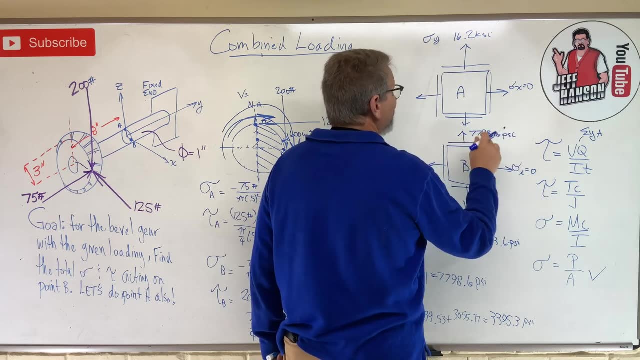 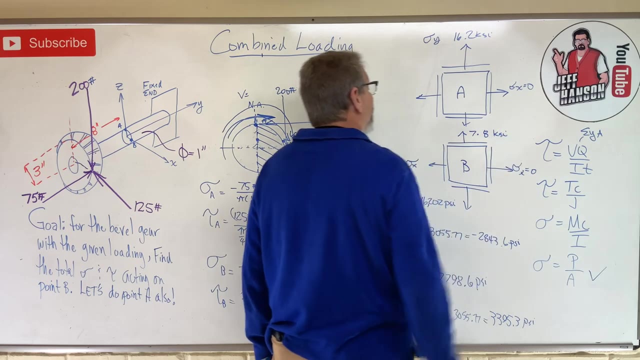 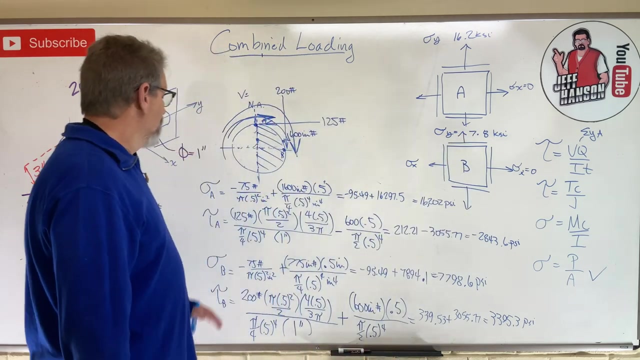 this guy is: uh, what do we say? 77, 98.6? or we could say, oh, let's do it like the other one. how about 7.8 ksi? okay, and that is my sigma y. okay, for for point b. now let's talk about tau stress, okay. so if we look at, 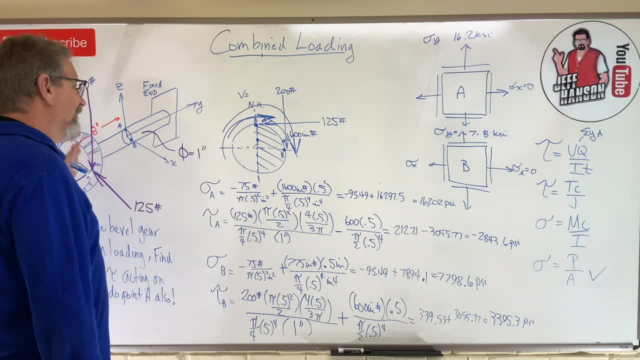 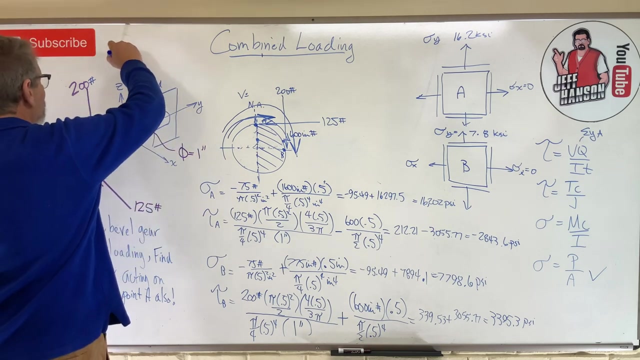 point a? okay, who made the shear for point a? the 200, right? no, point a, uh, who made the shear for a? uh, where is he? the 125, okay, so the 125.. so if i look straight down this beam like this, here's what the beam looks like. oh, let me draw it like this. this is so confusing y'all. 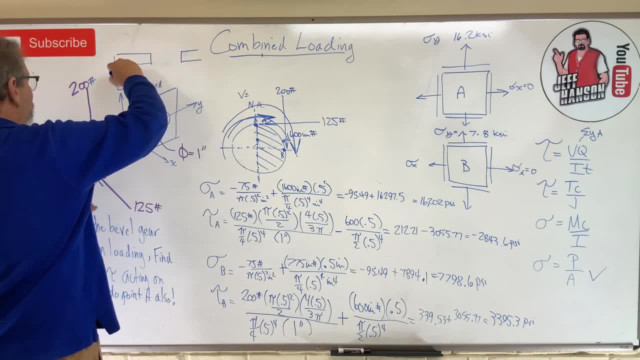 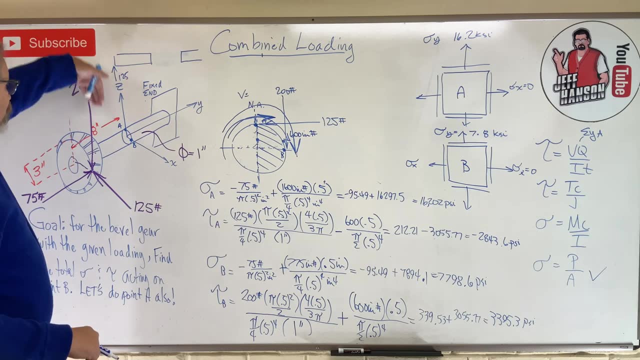 okay, here's the 125.. okay, so this is looking like straight down on the beam. if your eyeball is looking straight down the y-axis, what would you see? i would see this with the 125 pushing on me. here's my little stress element, right there. right, here's how you find the direction we know. 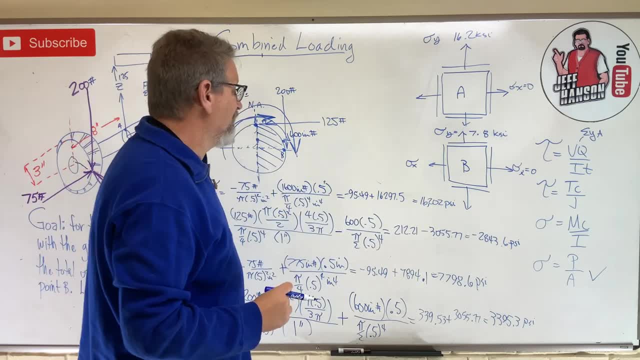 how big the shear is. it's twenty eight, forty three point six. twenty eight forty three, which is gonna be, let's just call it the 125.6, which is gonna be. let's just call it the 125.6. 28.63, which is gonna be, let's just call it the 28.53. 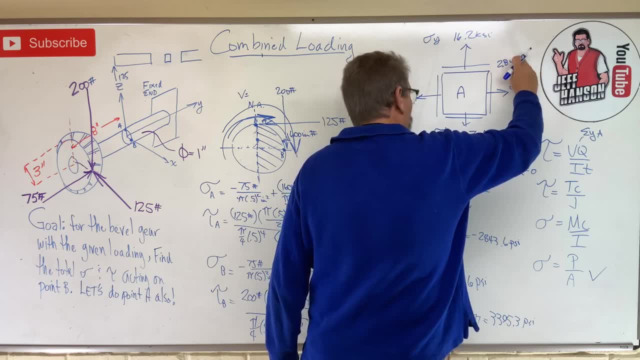 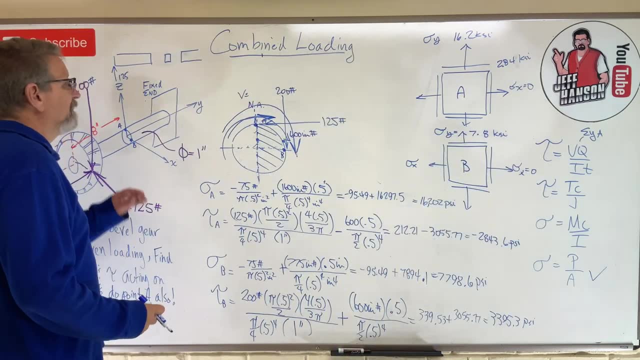 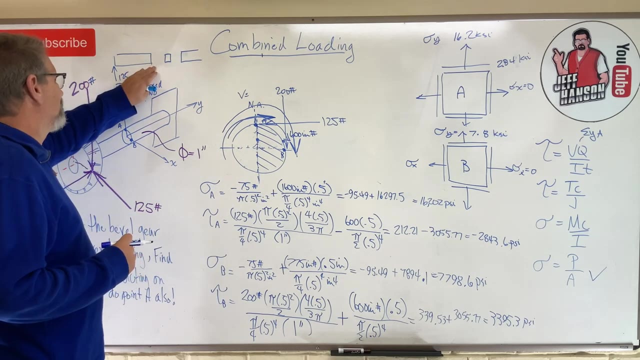 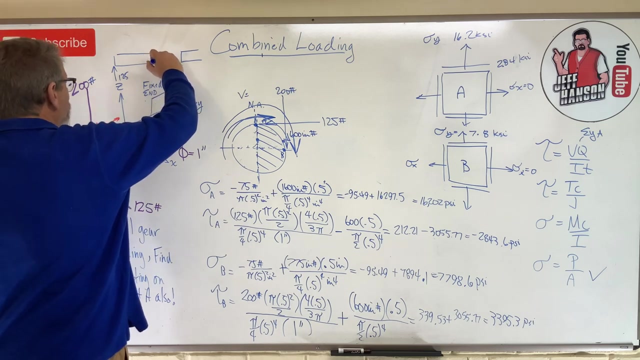 call it 2.84, 2.84, ksi. but which way do the arrows go? okay, so, which way the arrows go? so, on the Y face. on the Y face, because I'm looking at the Y face here. okay, this goes this way, this goes this way. so then my little stress element has: 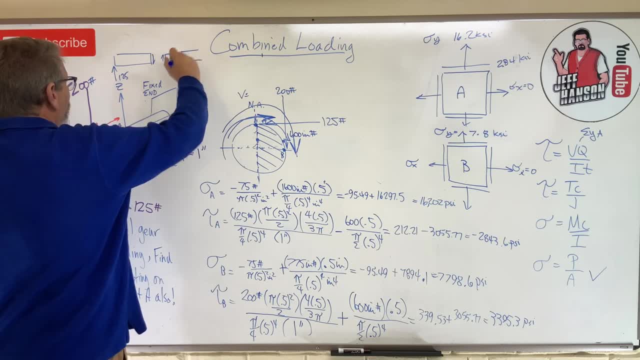 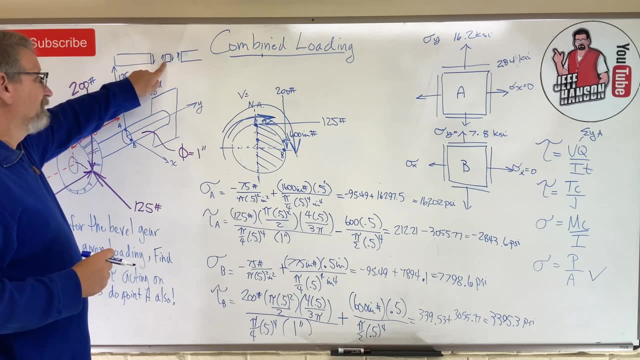 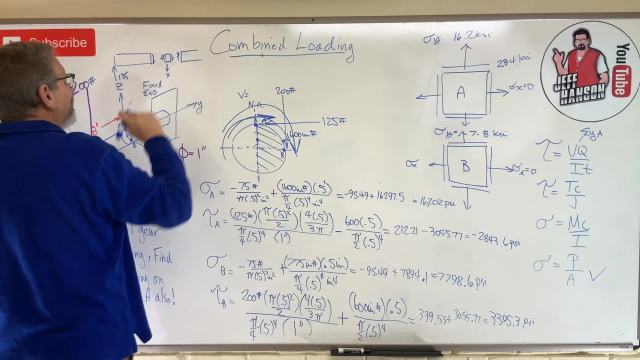 to be like this: doesn't it okay? if the 125 goes up, the next place is down, the next place here, okay. which means that that Y face- because here's, this is the X direction, okay, this is the Y direction. so the Y face has to go up on this side. 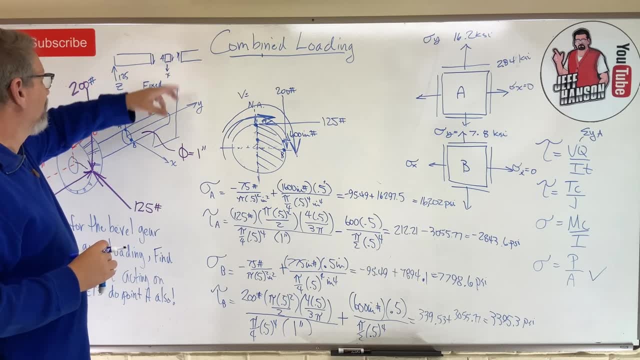 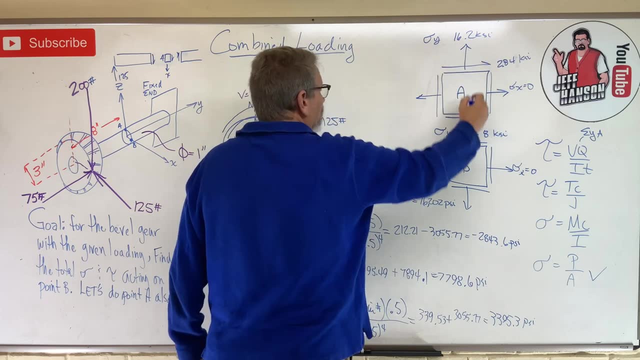 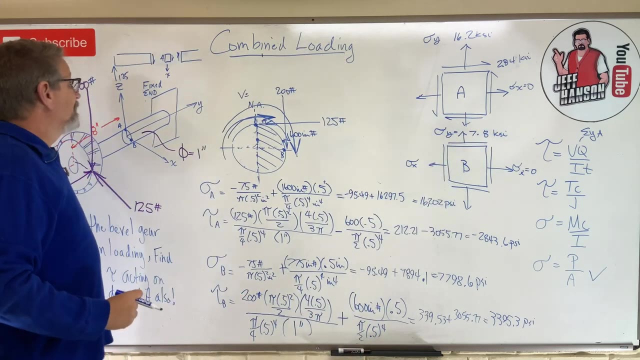 and down on that side, right? so if I'm looking at that, it's gonna go this way, right, yeah, and then this, it's got to go that way, this has got to go that way, it's gonna go that way, okay, gosh, that's confusing. I hope that. 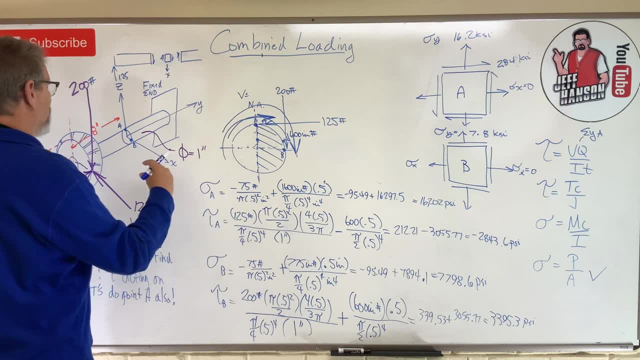 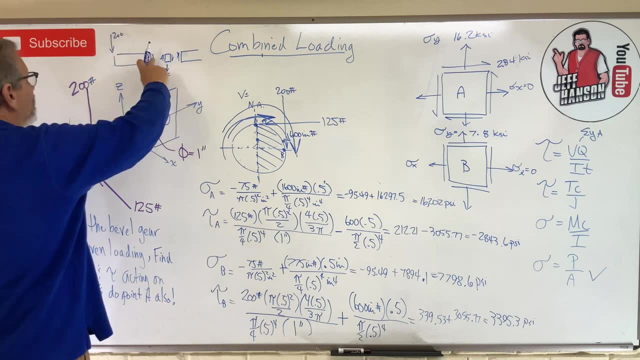 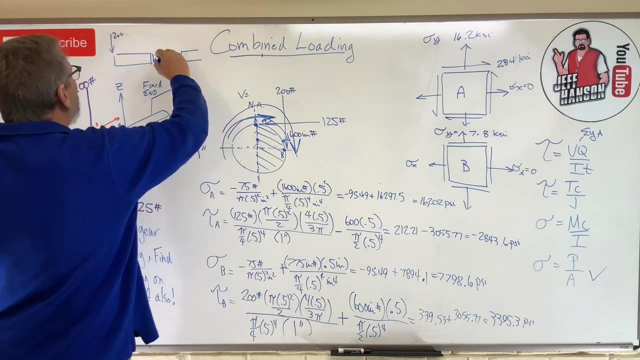 makes sense to you. if I'm looking straight on at B, I'm looking down the x-axis, right, what do I see? well, I see the 200 doing this. the 200 okay. so what does that mean? on the X, right in the Y direction, on that, that, on point B, it's. 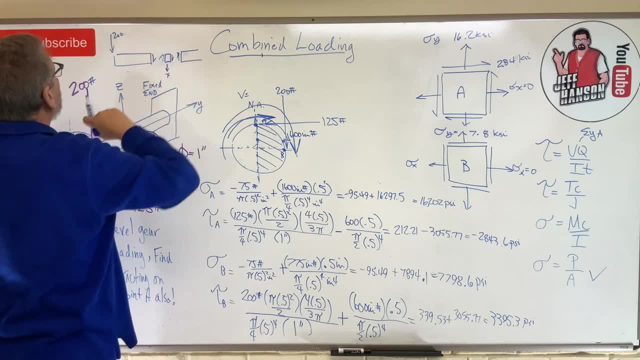 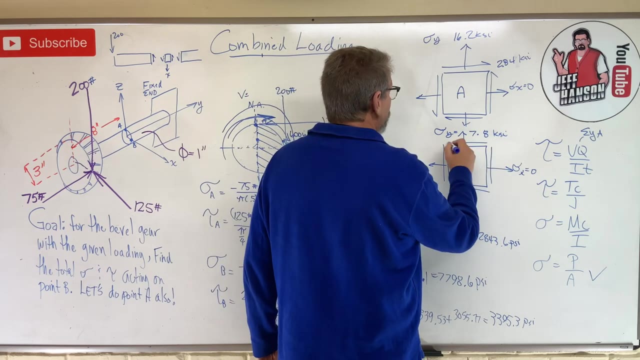 going to go that way or B going to go there? yeah, that's gonna make sense to you, going exactly the opposite direction, as it was there Down, it's got to go up, Up, down, up, down, right. So on B, it's going to be exactly the opposite. it was on A, So it's going to be over.